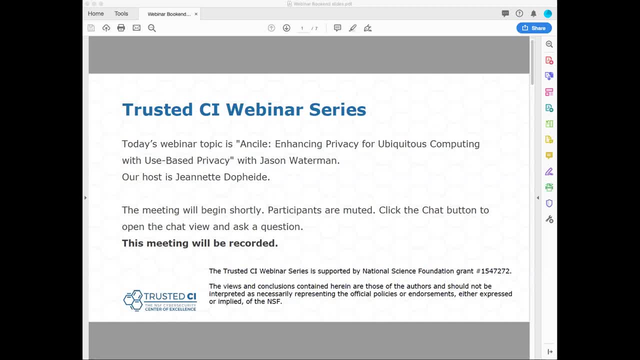 regarding cybersecurity to the NSF community. More information about Trusted CI can be found at TrustedCIorg. Today's topic is ANCEL: Enhancing Privacy for Ubiquitous Computing with Use-Based Policy with Jason Waterman. Jason is an assistant professor of computer. 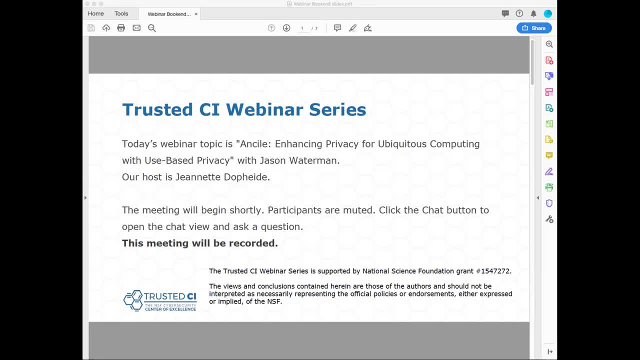 science at Vassar College. Before we begin, I have a few items to note. First, this presentation is being recorded. Second, participants are welcome to ask questions during the session using the chat box, And you just click on the chat icon and a little window will pop up. 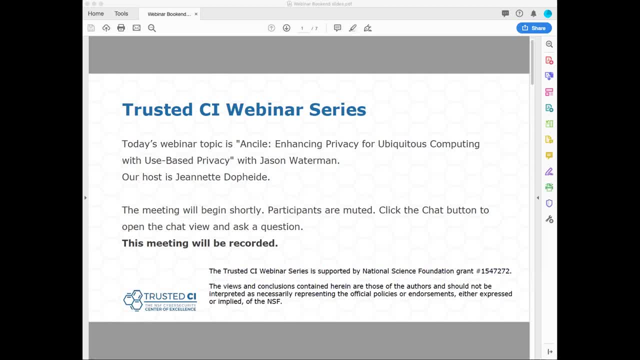 And we're going to be talking about how to use the chat box to ask questions during the session, And we have planned time at the end of the presentation to take questions as well, And with that I will hand the presentation over to Jason. Jason, welcome. 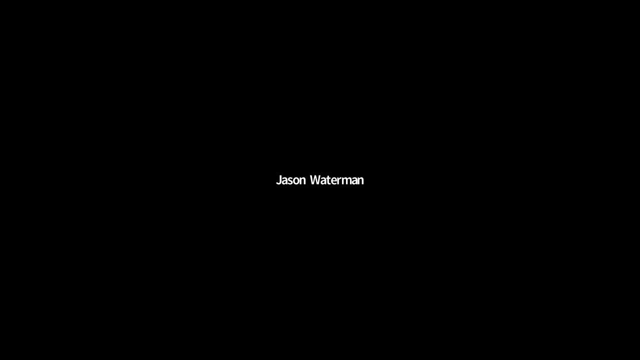 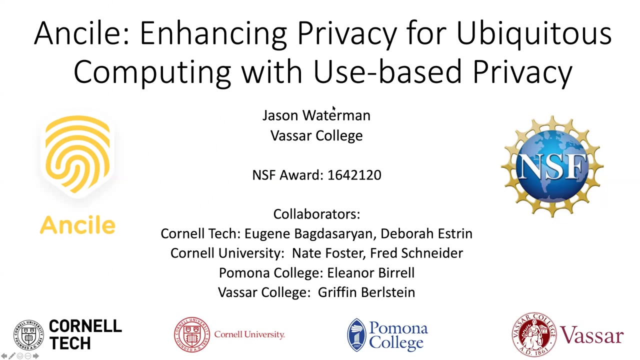 Great, thank you. All right, let me share my screen here. Great, Can everyone see that? Yep, you look good, Fantastic, Great. It's great to be here today to talk about ANCEL, our framework for developing privacy-aware ubiquitous computing applications. 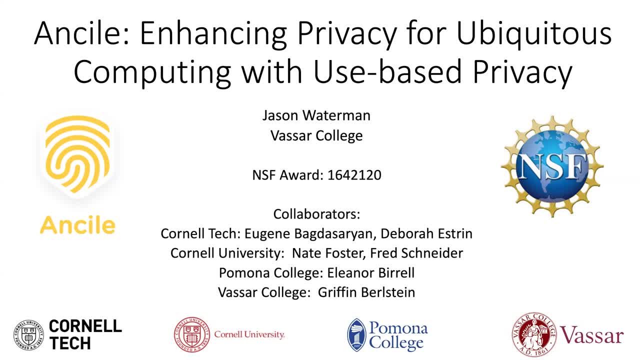 I'm Jason Waterman from Vassar College. I'll be giving you an overview of our system today, but this project is truly a team effort. From Cornell Tech, we have Eugene, who is a PhD candidate and is being supervised by Deborah. At Cornell University, we have Nate and Fred who oversee. 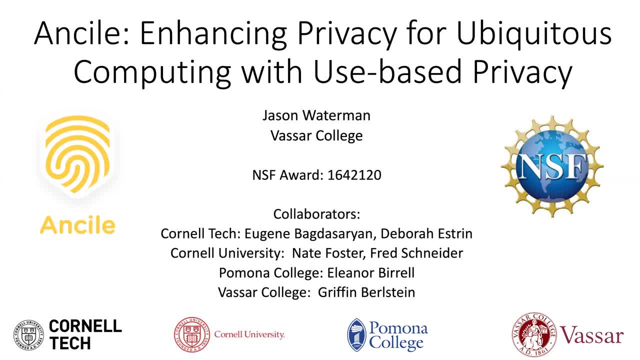 the project And Eleanor at Pomona College, recently received her PhD, with Fred acting as her advisor. And Griffin is my student, who, of course, is going to be working with me on the next session student who graduated from Vassar in May. 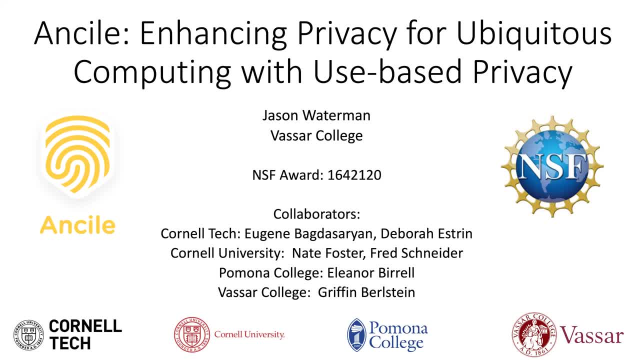 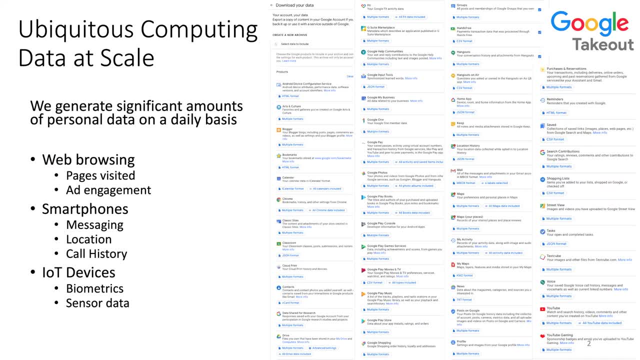 and I'm proud to say he will be starting his PhD at Cornell University this fall. So the recent proliferation of sensors have created an environment where our behaviors are just, are being continuously monitored and recorded, And that data is very personal to us, For example, fine-grained location data. 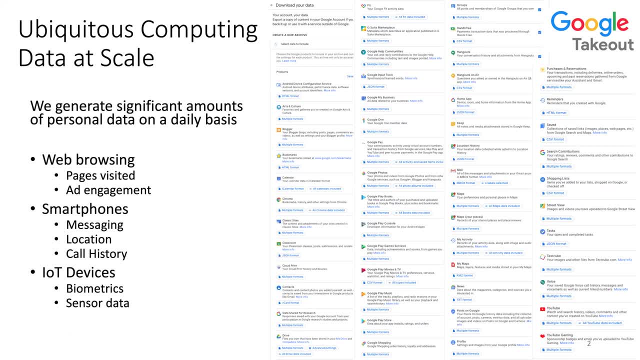 is being generated wherever we carry a phone. For example, Google Takeouts, a service that lets you download your data. collected by Google, shows a staggering number of things that they collect about you, And this is just one of the many service providers that we interact with on a daily basis. 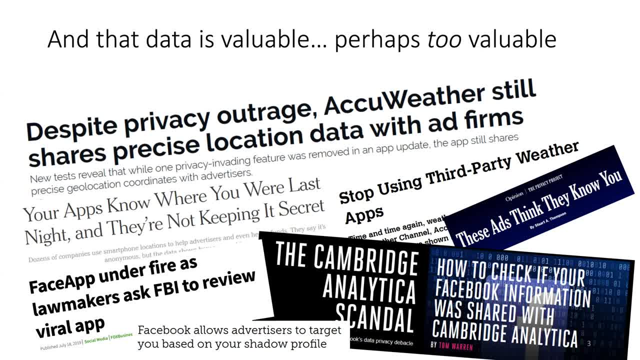 And they collect that data because it's valuable. It doesn't take too much internet searching to find numerous examples of where companies arguably have crossed the line with regards to social norms. AccuWeather, a weather application which uses your location to show you the weather in your area, which makes sense. 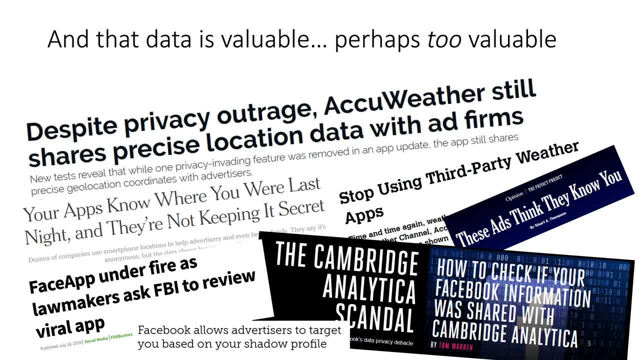 collects your location data and sells it to third-party advertisers, even when you're not using the application. And making headlines from just a few days ago: FaceApp, an application where you upload a picture of yourself and it shows you an aged version of your shelf. 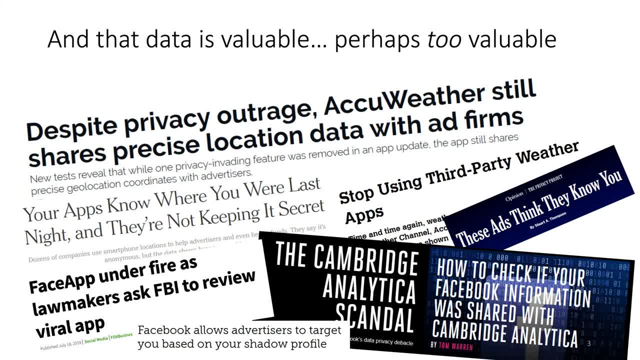 or there's other sort of transformations that you can do. it went viral, But if you look at the terms of service, it raises some privacy concerns About what they do with your image once you've uploaded it, And the larger concern here is that even if they're 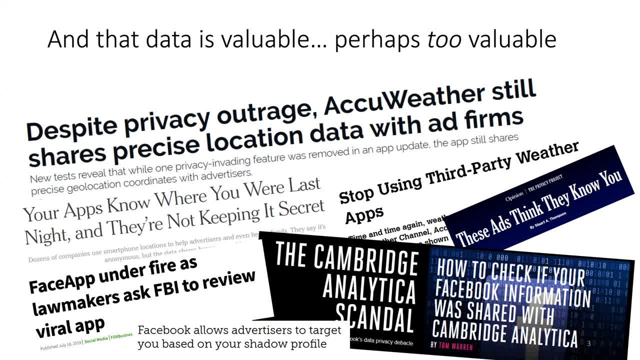 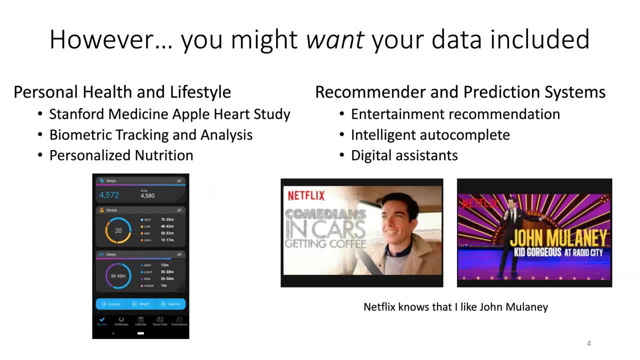 kind of acting on the up and up with our image data. we really have no way of knowing exactly what they're doing with their images, But for many reasons, there are many reasons why we want to share our data. Health and wellness applications can nudge us. 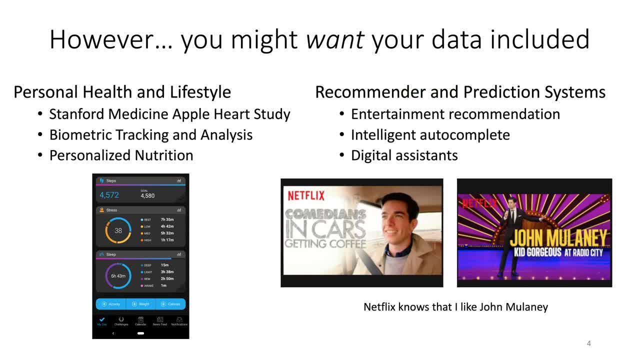 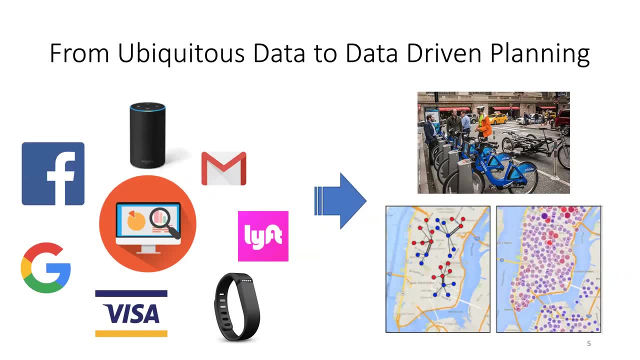 into making healthier life choices and recommender and prediction systems. It can help us decide what to listen to or watch on a Friday night. And, aside from our personal data, when we put data being collected at scale, it can lead to solving an array of space management. 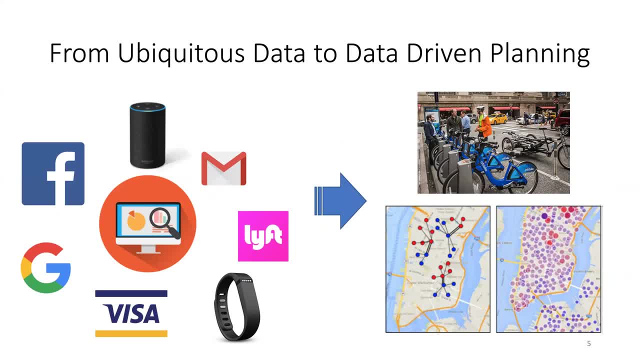 and sharing needs. The images on the right show one example of data-driven planning. This is the Bike Angels program, which uses real-time tracking of CityShare bikes to build models that reward users who move bikes from more congested areas, as you should kind of see in the image on the lower left-hand. 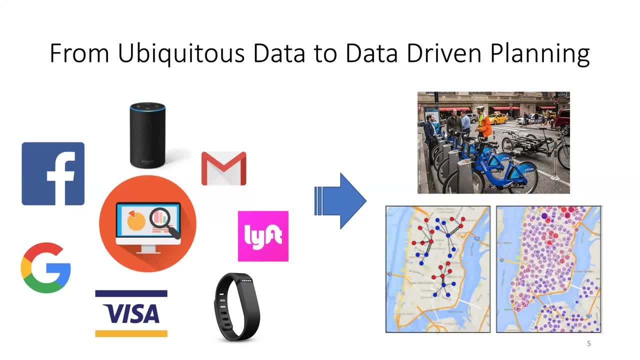 image where they move them to congestion areas to less congested ones. So this saves the trouble and expense of manually moving these CityShare bikes with either trucks or you can see a picture on the top right of these tricycles that manually move them. 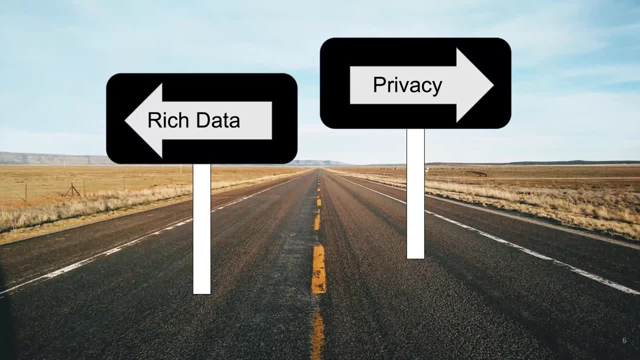 So it's clear that the data is useful for a wide range of applications, but there's clearly this tension between an application's desire for rich data and a person's willingness to trust that application with their data, And so I argue that it requires a system architecture. 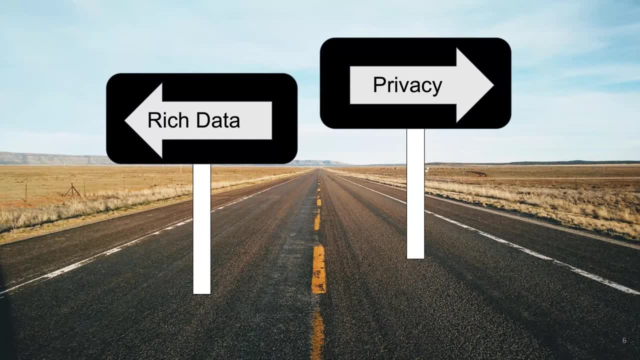 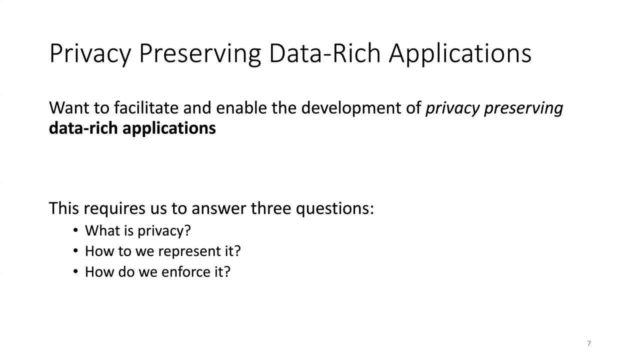 and a framework that supports policies, privacy policies- as first-class primitives, And our system, ANSILE, is a framework that provides this support. So ANSILE supports the development of privacy-preserving data-rich applications. To see how this is done, I'd like. 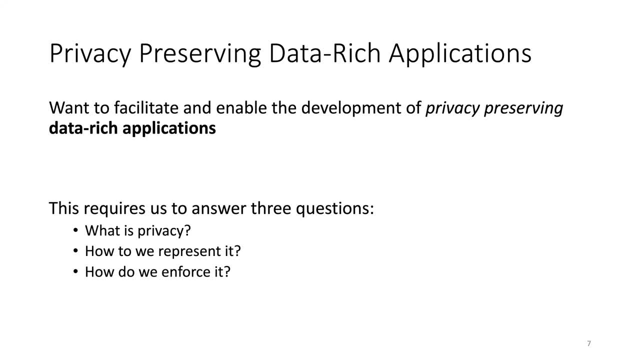 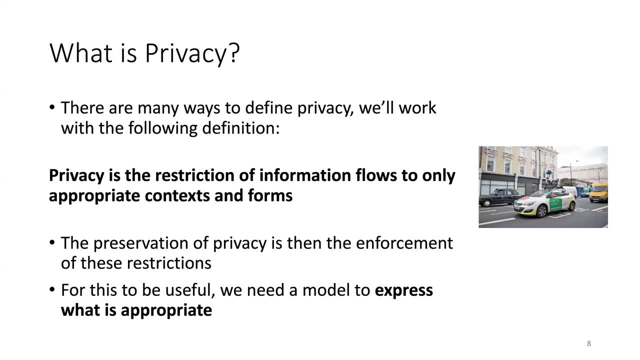 to answer three questions. First, what is privacy, How can we represent privacy in our system And, finally, how can we enforce it? So first, what's privacy? There's lots of ways to define it, but we'll go with the following definition. 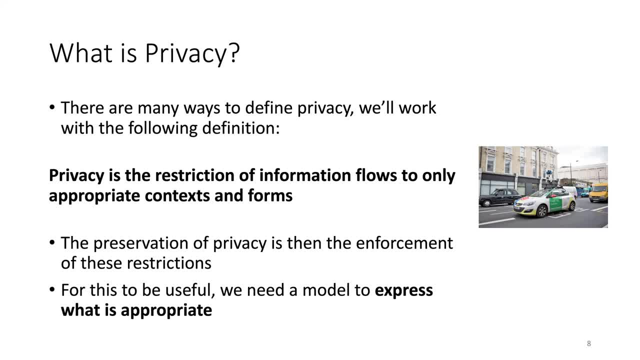 Privacy is the restriction of information flows to only appropriate context and forms. Take Google Street View, for example. Am I comfortable with a Google Street View car taking a picture of my house once a year to improve Google's Maps? Sure, Why not? 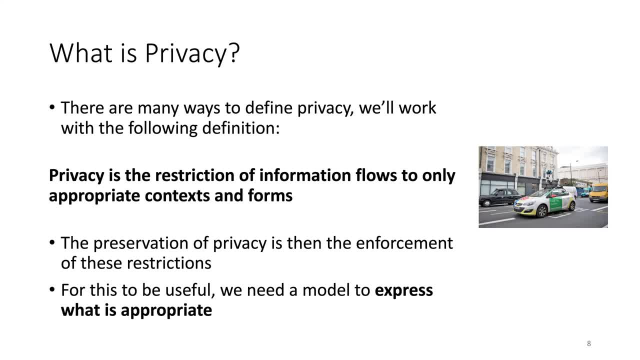 That sounds like a good cause. However, would I be comfortable with that same car parking outside of my house streaming a video feed of my house to YouTube? Absolutely not, And so context here really matters, And Our definition is that my privacy is preserved. 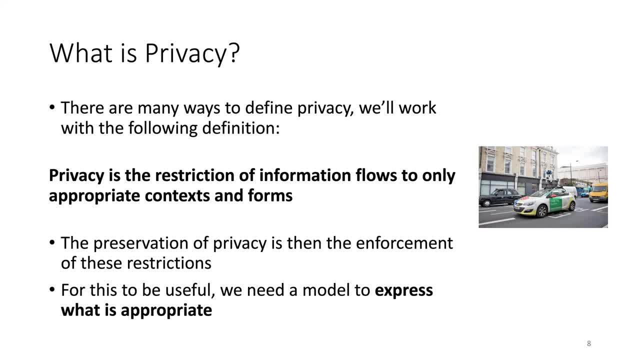 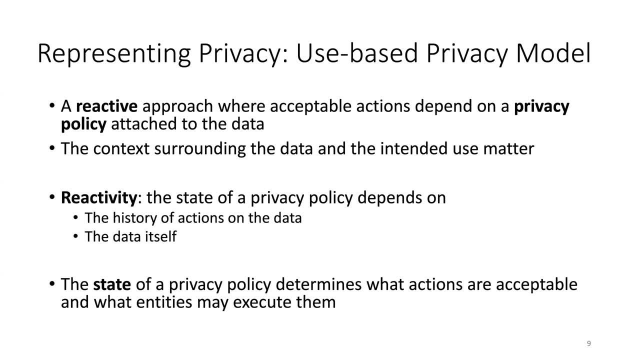 when I can express what's appropriate or not and have those restrictions enforced. So how do we represent privacy? One model that can help us is use-based privacy, where we define, where acceptable actions depend on the context surrounding the data and the intended use of that data. 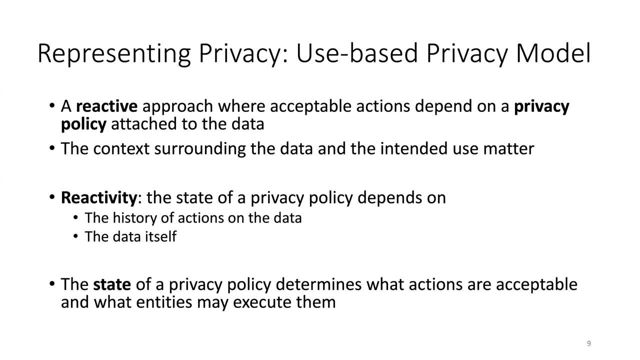 So use-based privacy models are reactive And the state of what is allowed depends not only on the data itself, but the history of the actions on that data. The current state of the policy determines what actions are acceptable, And let's take a look at an example of use-based privacy. 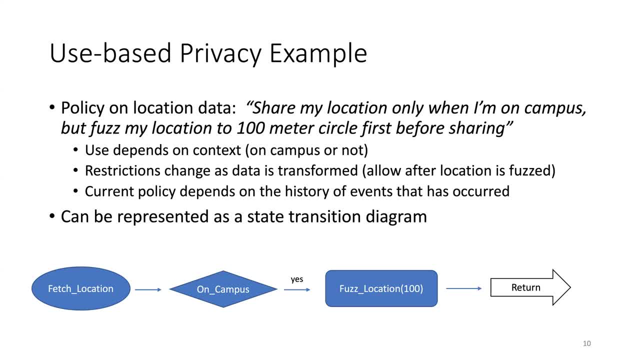 For this example, we have a policy on location data And for this policy I'm OK sharing my location If I'm on campus, But I'm not exactly comfortable sharing my exact location, So before I'd like to share my application. 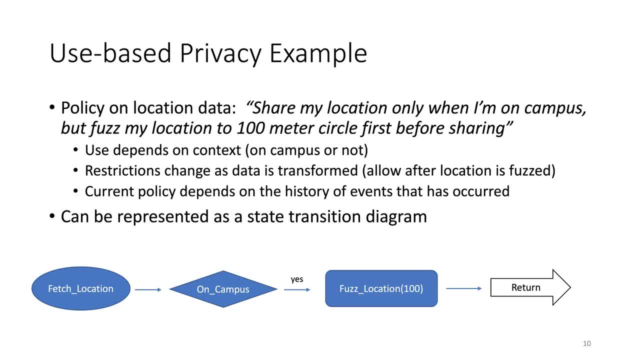 I'd like some noise added to my location to fuzz it to a region of uncertainty of about 100 meters. This should give people enough detail to know which building I'm in on campus, but not at the office level detail. So this example shows that my permitted use depends. 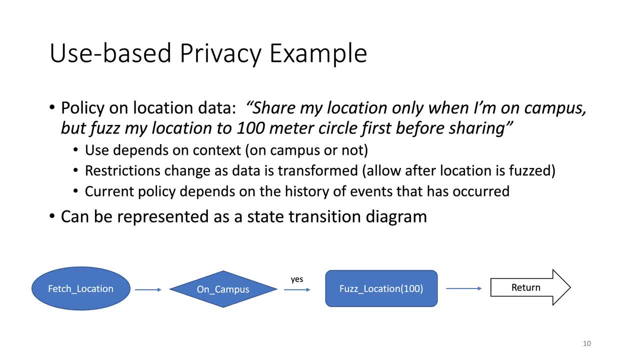 on context, whether I'm on campus or not, And it shows that restrictions on data change based on transformations of that data. In this case, I will allow my fuzz data to be shared, So these set of possible use authorizations forms a finite state automaton. 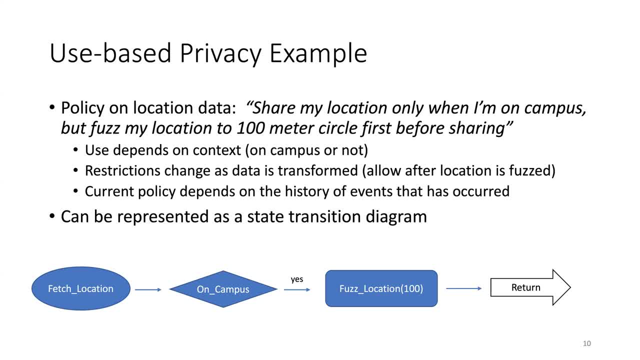 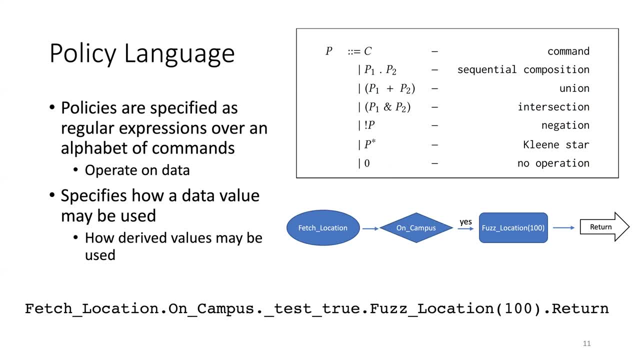 And the state of this privacy information changes when events, either environmental events or transformation events, occur. So formally in our system, policies are specified as regular expressions over an alphabet of commands. These commands operate on data And the regular expression specifies how. 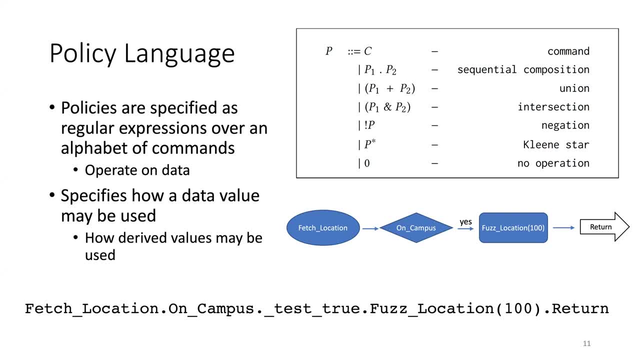 a data value may be used. Our policy language supports the normal standard operations on regular expressions And I've shown them in the upper right corner And the state transition diagram shows our example that I described on the previous slide, And on the bottom is that state transition diagram represented. 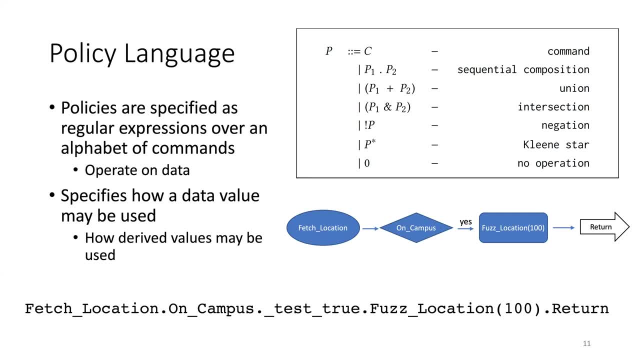 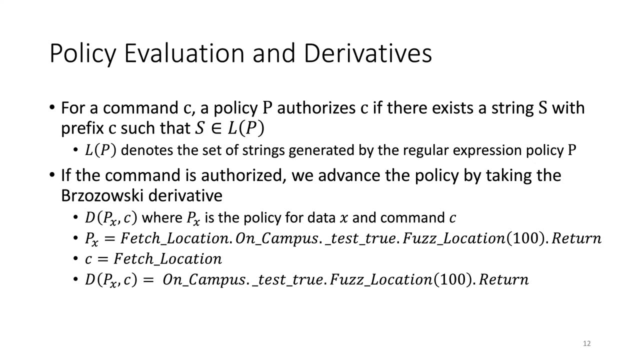 as a regular expression, The command that comes after the on campus, the underscore test. true, this is an internal ANSILE command that's used to support policy branches, And I'll talk a little bit more about this later. So we can evaluate. 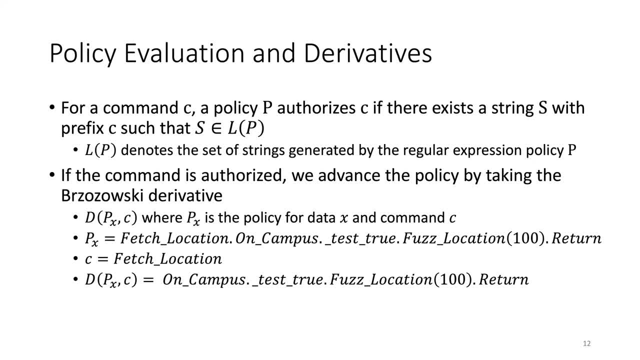 The policy regular expression to see if a given command is authorized or not. Formally, for command C, a policy P authorizes that command if there exists a string S with the prefix of C, such that the string is in the set of strings generated by the regular expression P. 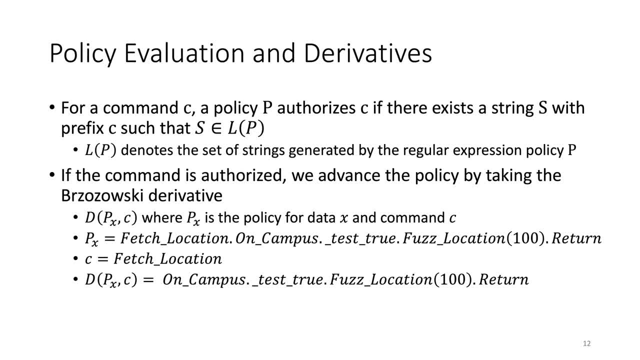 In other words, if our command is a valid prefix in the set of strings that that policy can generate, we will authorize that command. If that command is authorized, then we're going to advance that policy by taking the derivative. In our example, P sub X is the policy at the start. 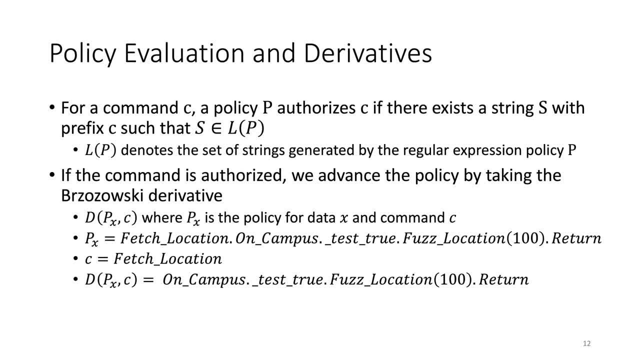 The command C, fetch location, is authorized because it's a valid prefix of P sub X. Our system will check and then, when it's authorized, we'll execute the fetch location commands And the new policy is going to be the derivative for this example. 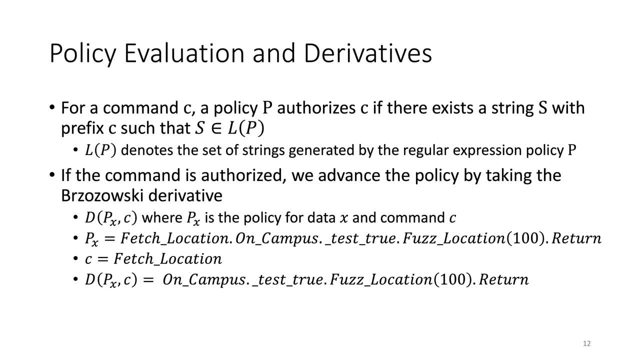 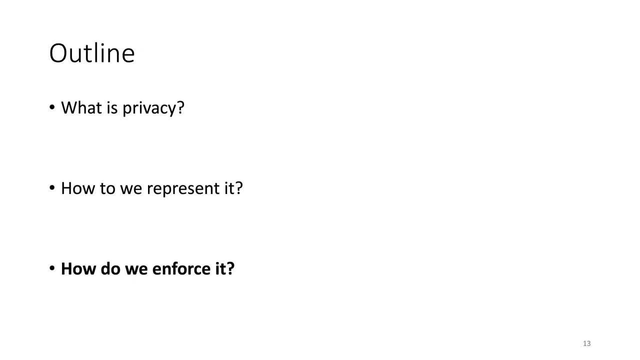 it's going to be P sub X, with the prefix fetch location removed from there. OK, so kind of where are we so far? So we've described privacy as the restriction of information to only appropriate contexts and forms, And we've seen that we can represent policies. 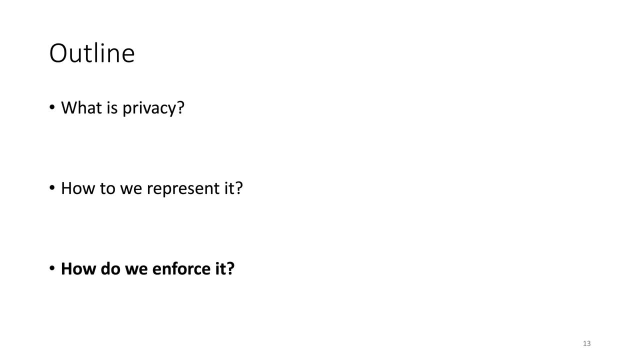 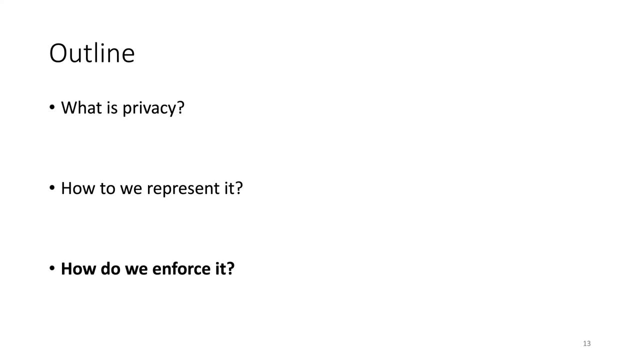 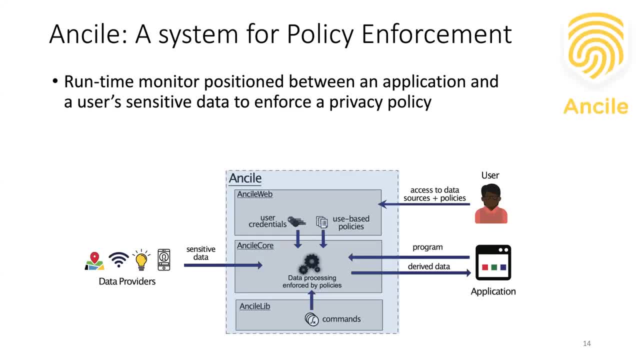 So let's get started. ANSILE is a runtime monitor positioned between an application and a user-sensitive data, And the goal of ANSILE is to enforce a privacy policy. We get the name ANSILE from because in ancient Rome, 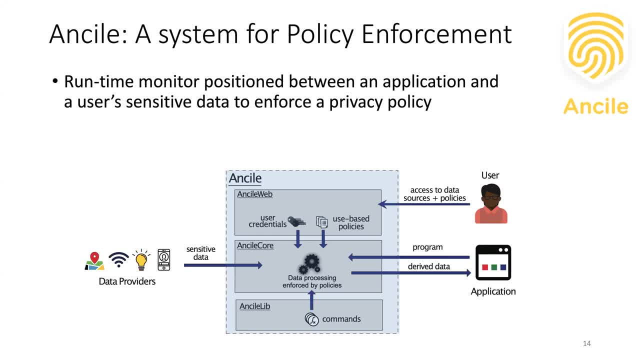 an ANSILE was a sacred shield. The legend is is that they were a set of these 12 shields, And one of these shields fell from heaven, was seen as a token guarding the Roman Empire. So in this way we view our system. 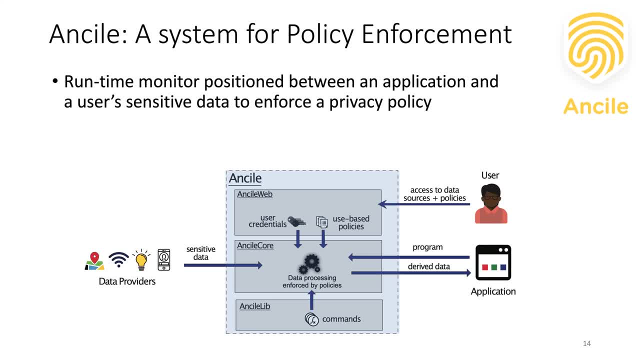 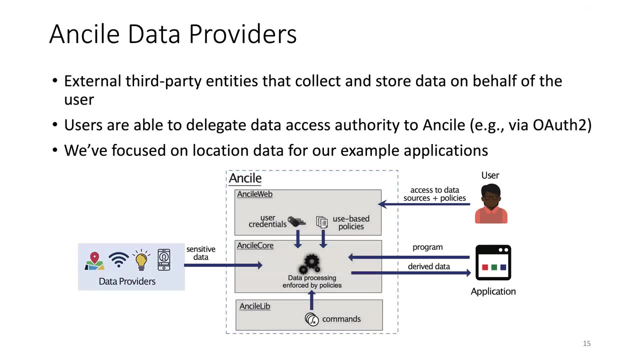 as a shield protecting the privacy of a user's data. Before we describe ANSILE in detail, I'd like to talk about the three main entities that interact with ANSILE: data providers, ANSILE users and applications. Data providers are external. 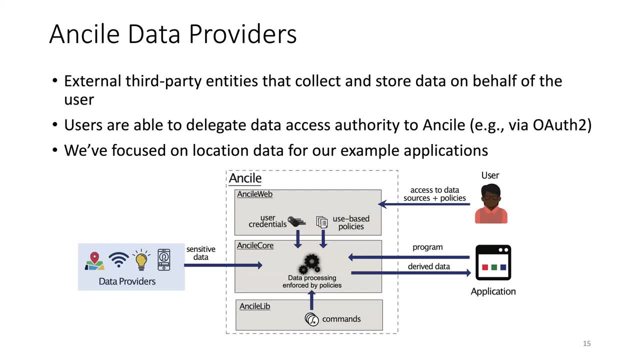 entities to our system. They collect and store data on behalf of the user. We also assume that users are able to delegate data access authority to ANSILE through a mechanism such as OAuth2.. For the examples I'll talk about today, I focus on location data because I think that's a good proxy for the challenges. 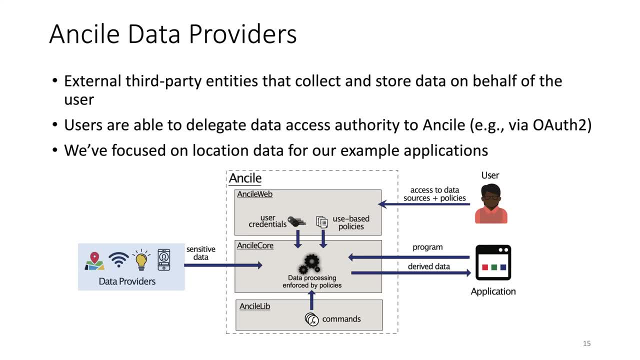 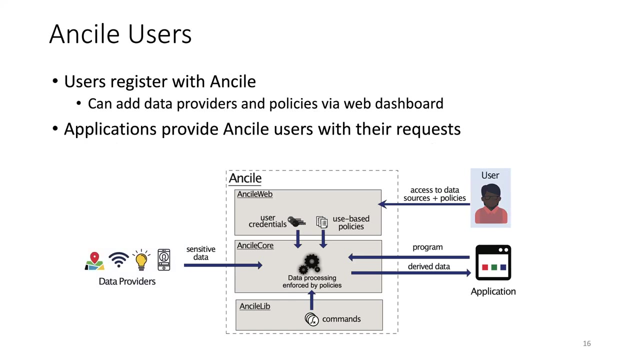 that arrive in ubiquitous computings in general, and it's kind of obvious that location is a pretty sensitive data to be collected. So our applications kind of focus on location based. but ANSILE can work with any OAuth2 protected data source Before users can before. 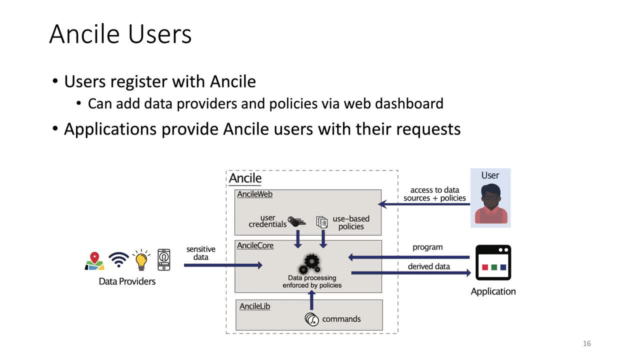 anyone can use an ANSILE application. users must first register and create an ANSILE account. Once they've registered, We have a dashboard, which I'll show you what that looks like in a second. They can add data providers, so they can kind of hook up data providers. 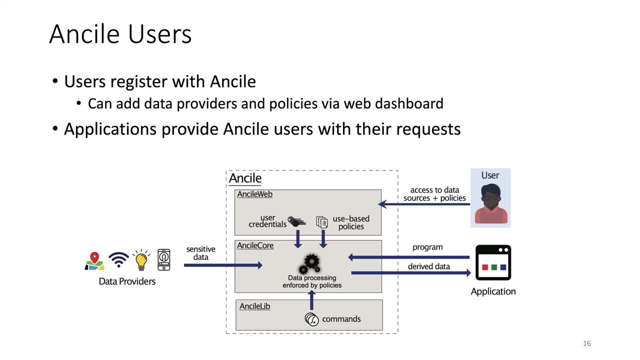 And along with those data providers, they can provide policies, And I'll talk about what those look like in a minute. When ANSILE applications make requests- any requests to the system, they must provide one or more ANSILE users with that request. 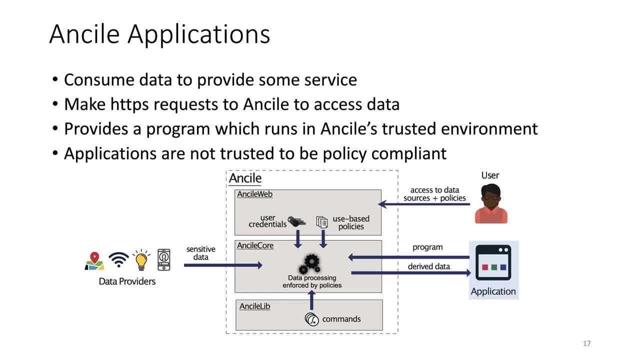 And the last entity that I want to talk about that interacts with ANSILE are applications. Their job is to consume external data and provide some service by making requests to ANSILE. In the request, the application submits a program which runs inside of ANSILE's trusted environment. 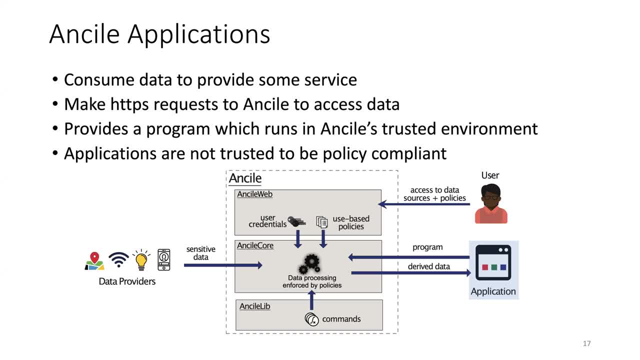 Inside of that environment, ANSILE will get the data from the data providers and perform computation on that data. We don't assume, we don't fully trust the application In that we don't assume that the program that the application submits to run inside of ANSILE is policy compliant. 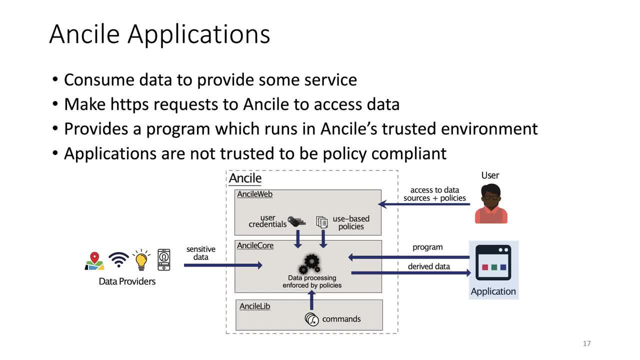 And so when that program is being executed inside of ANSILE, it's checked in real time by ANSILE's runtime monitor. We do, though, kind of assume that the applications don't try to actively try to find and exploit vulnerabilities in the system code. 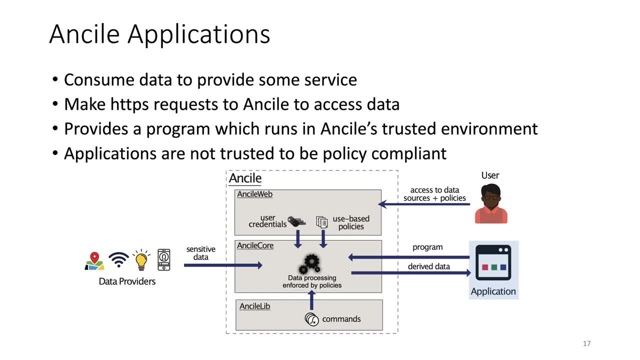 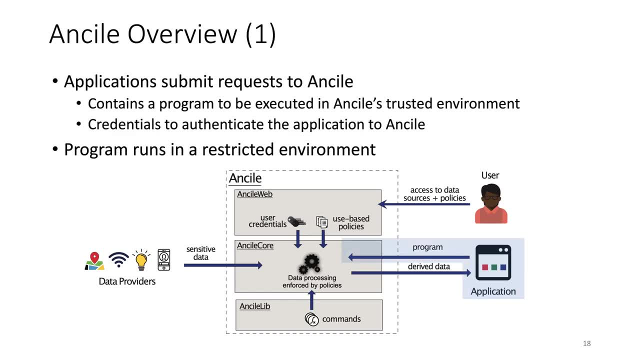 And that they don't try to perform denial. So there's the question about ANSILE being a service-based institution. Okay, So now that we've talked about the entities that interact with ANSILE, let's go through a life cycle of an ANSILE request to get a better overview of what the system looks like. 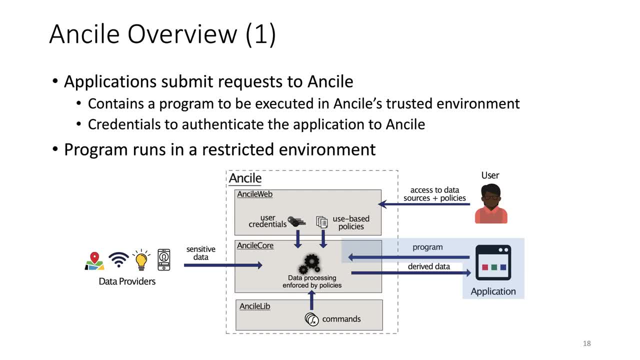 Applications submit request to ANSILE. The request contains a token that ANSILE uses to authenticate the application to ANSILE, So we know that what application is performing and using it. We also know the number of files and networks that are being used. So we know that the application is performing a request to ANSILE, And then we know the application is performing a request to ANSILE, And then we know that the application is performing a request to ANSILE, So we know the application is doing what the application does. 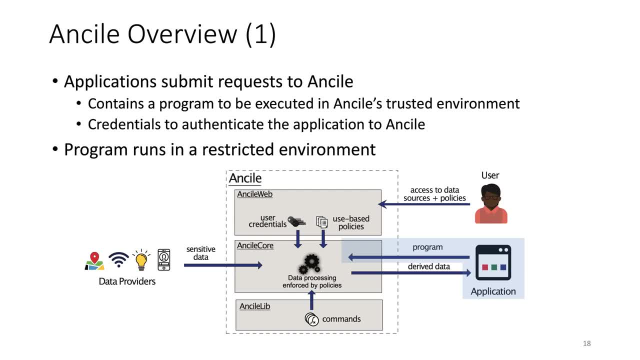 So for those who are trying to run in the system, they're using the same system as well, asking for services, And the request also comes with one or more users that the request is for, and the program will execute in a trusted environment. Okay, so once the program has 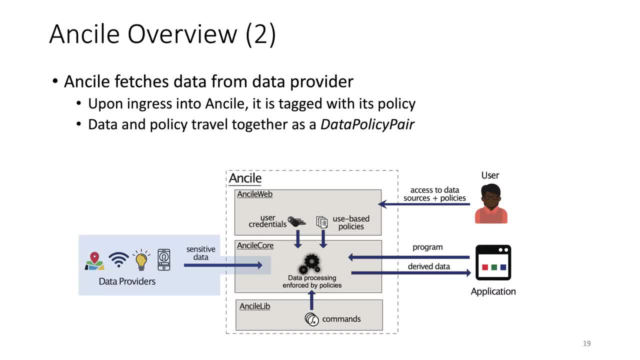 been submitted, Antile will start executing the program, and programs start by calling a command that fetches data from some third-party data provider, And so when that data enters into Antile, it's immediately tagged with its corresponding policy And the data and policy. 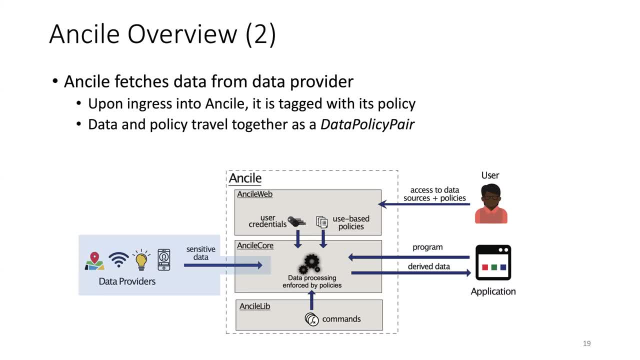 are joined together as a data policy pair object. This data policy pair is one of the key programming abstractions in Antile and we'll see some examples of that later. So once we have data that's entered into the system and it's been tagged with its policy, Antile executes the 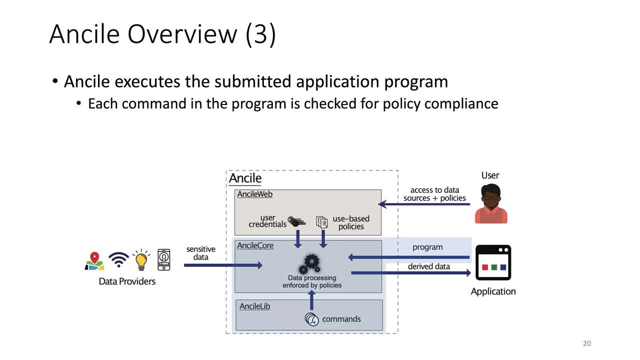 rest of the submitted program. The only way to access the data is through privileged Antile commands. Each of these commands are checked for policy compliance before execution. So Antile will run the program and, if authorized by the policy and if all of the commands in the program were authorized, any derived output. so if the data has been, 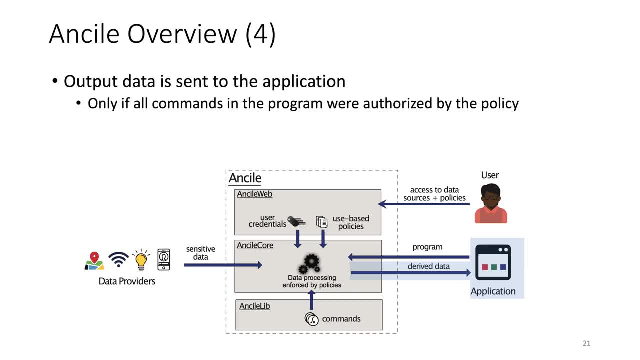 transformed, any derived output can be sent back to the application, And so once that data leaves the trusted environment of Antile, we don't make any further guarantees about how that data can will be used. So once it leaves, all bets are off. And then finally, when the program finishes, 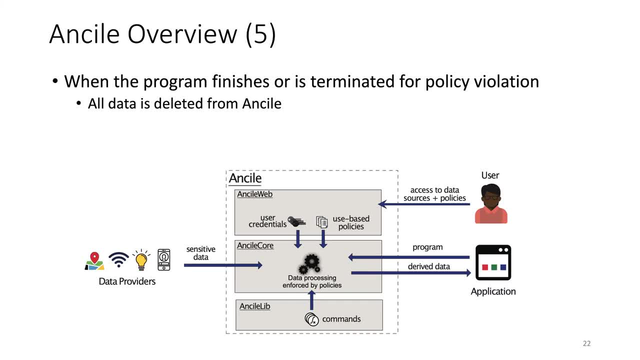 execution inside of Antile or is terminated by Antile for a policy violation, all data associated with that request is deleted from Antile. And so no data, no data from external data providers is stored inside of Antile, outside of the execution of that program. So once the program terminates, 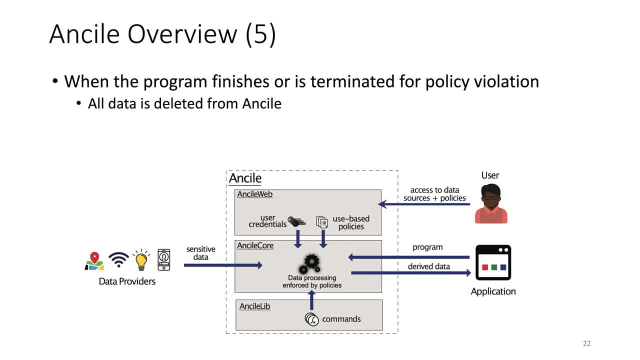 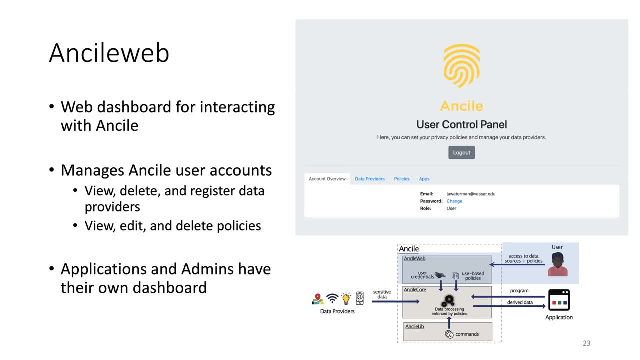 that data is no longer kept inside of Antile. Okay, so now that we've kind of gone over our data, given an overview of the system, we can kind of dive down and look deeper at the three main components of Antile. So the first one. we'll start with Antile Web first, And this is the user. 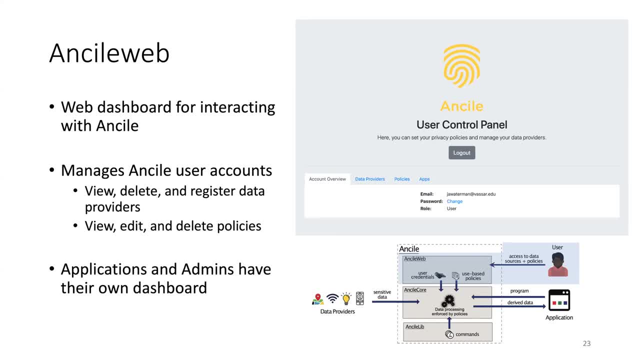 control panel for interacting with Antile. And so this is kind of when somebody wants to register for an Antile account and they want to see what data providers that they have registered and what policies associated with that, And so this is kind of when somebody wants to register for an Antile. 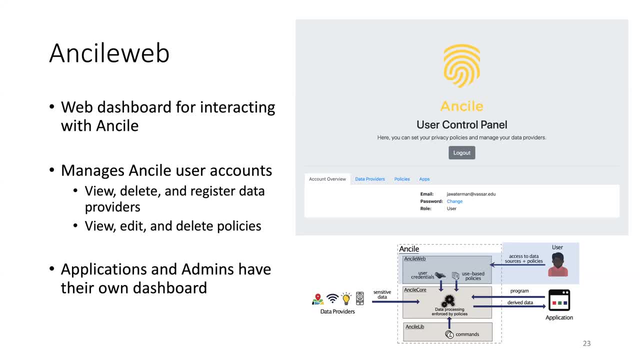 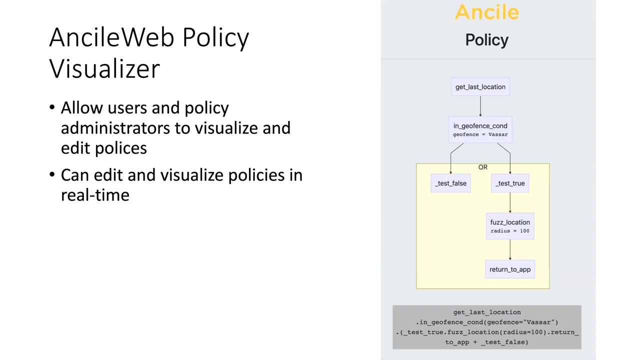 web. they can do this from this kind of web dashboard. In addition to a user control panel, applications have their own control panel and administrators have their own control panel as well. So one of the nice things about Antile Web is we have a policy visualizer- So regular. 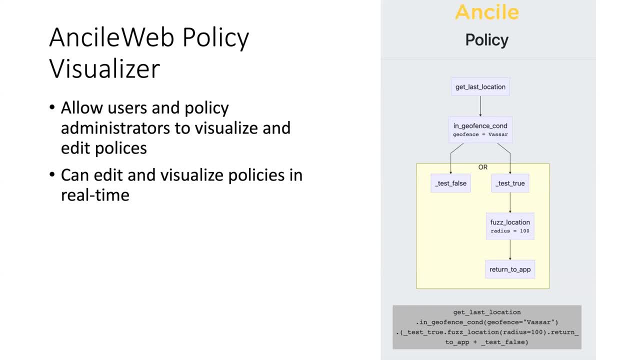 expressions are a familiar tool for most programmers, You know, and many of you. many of them are kind of comfortable operating with regular expressions, but for some more complicated policies it can be a bit hard to visualize. So what we've done is we've added a. 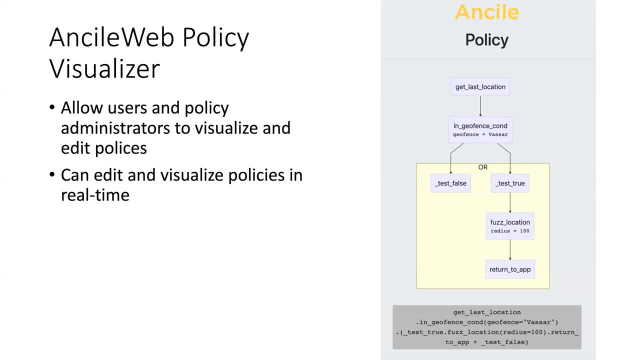 policy visualizer that lets users see a graphical representation of their policies and it allows policy administrators to visualize in real time the policy as they edit. So if you're kind of modifying a policy, it brings up a little text box and you can edit it and basically it sends. 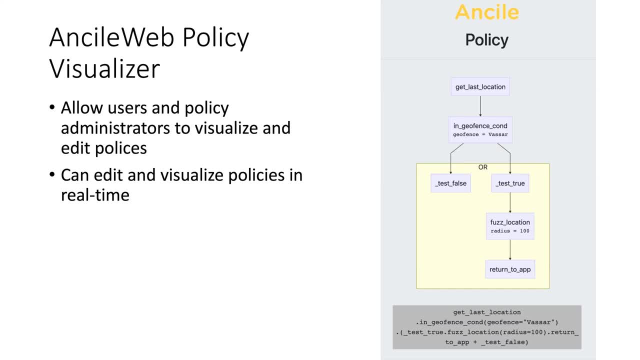 kind of that text box to the user, And so that's kind of what we've done, And then we've added a text box over to Antile that will parse the policy and then send it back so we can kind of see in real time what that policy looks like. And the policy I've shown here is the fully coded Antile. 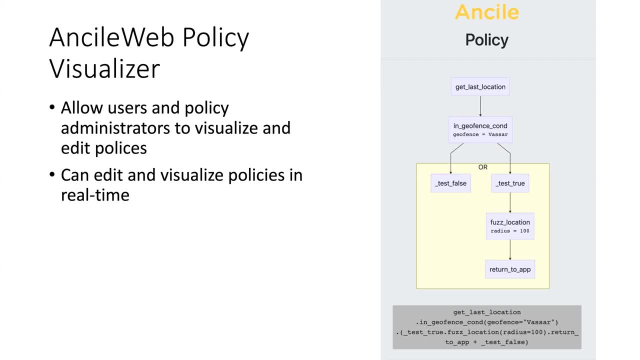 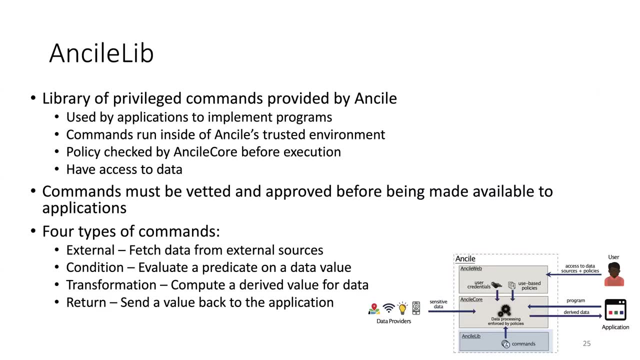 policy for the previous example that we looked at. The next component that I'd like to talk about is Antile lib, and this is the library of privilege commands provided by Antile Antile. As previously stated, these commands are checked for policy compliance before being. 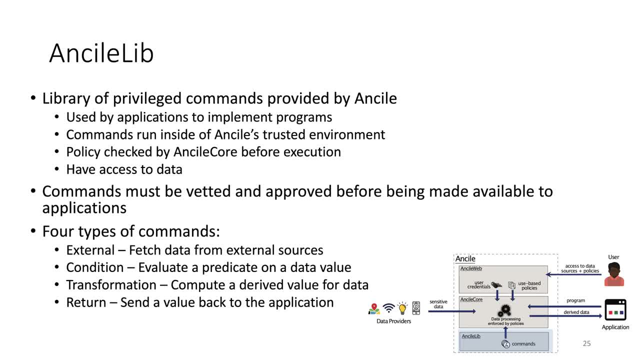 executed by an Antile program. and these privilege commands and what makes them special is that they have full access to the data and the policy associated with them, And that's why they're privileged. We provide a general purpose library of Antile commands, but applications can add their. own custom commands and they're also subject to a different privacy protocol. So the bread and butter provides that for everyone to do, and it's also- you know that's- a huge advantage of Antile, because they also provide you with free access to your own policy, to your login form, And so you. 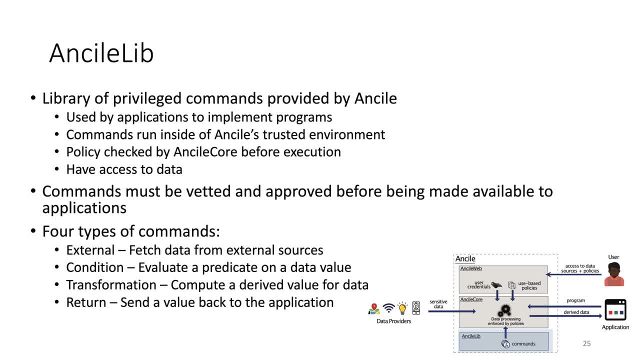 can also have access to all these commands that you use, And so what's interesting about this is. so how do I say that's a great thing If one of the if they need to do something that isn't already provided by our, our library? 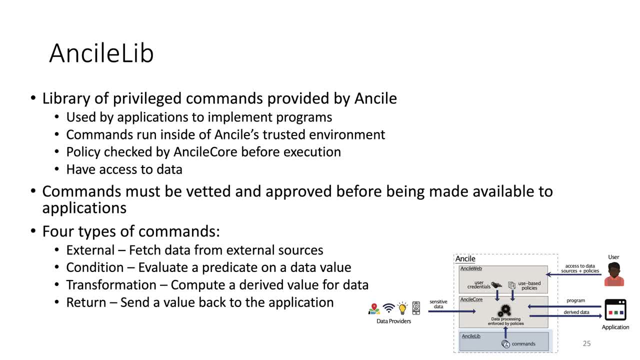 And as these commands are privileged, They have to be carefully vetted before being made available to the system. And so right now that process is a manual process where we kind of inspect the code To make sure that it's that it's not doing anything that it shouldn't be. 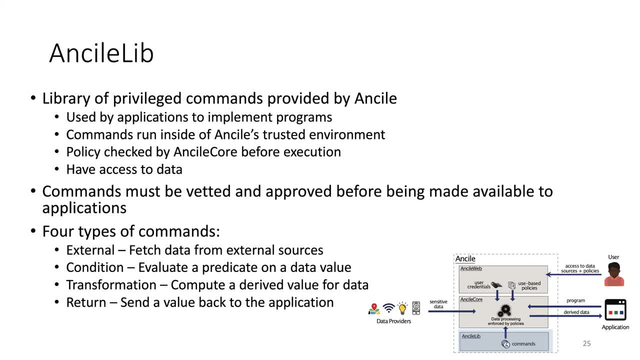 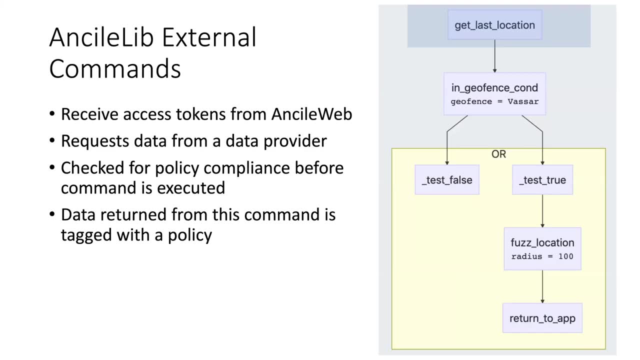 Before we Commit it to the system. There's basically four types of commands And n style lip that do slightly different functions, and I want to say a little bit about kind of each of them. next. so the first command That programs start off with our external commands. these external commands fetch data from external sources. 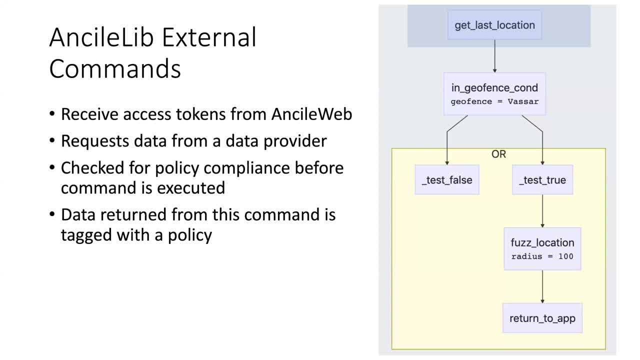 and so, as we saw kind of when I talked about in the Web part, when users connect to a data source to ancel, They can use kind of n-style web to authorize access to their data on their behalf. we currently support OH off to and Ant silo will store and manage these Oh off tokens on behalf of the user, and this is nice. 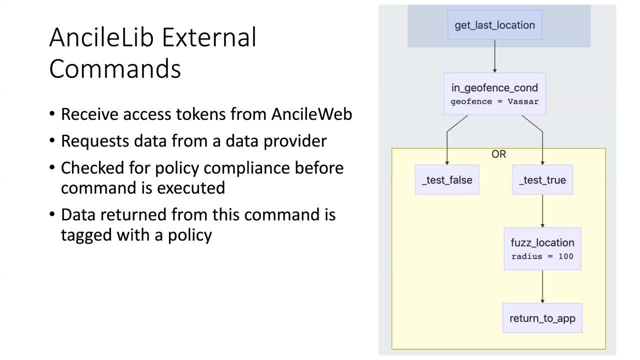 So the actual applications that make requests into n style. they never see these OAuth tokens. They're stored inside of n style behalf of the user for the application. so what that means is is that a user needs to be able to trust and style but the application, since those applications 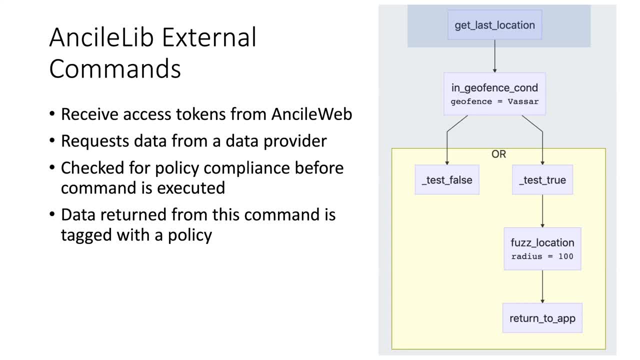 never see these authorization tokens, these Apple, these applications don't have to be trusted by the user. so as long as they trust and style, they don't have to trust the applications because those applications just never see those tokens. so, for this example, get last location. what that will do is that will. 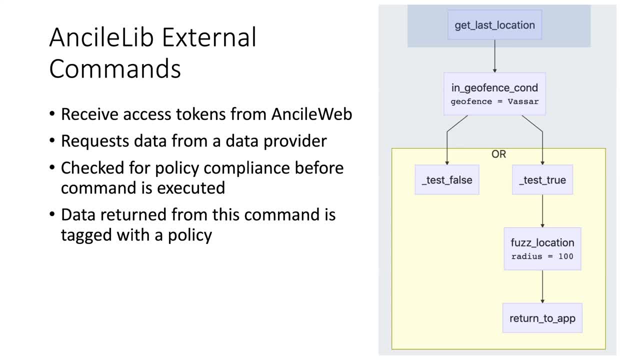 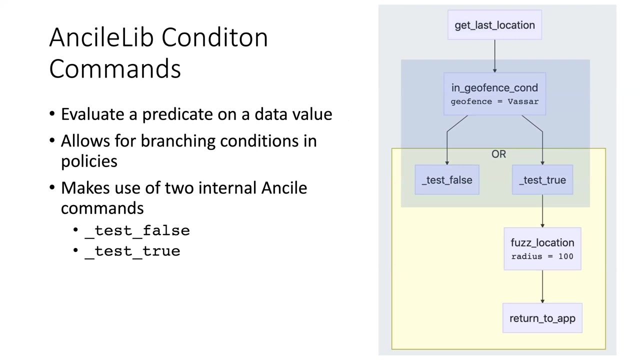 contact our location storage provider. we've built one locally for for our test beds and it will get the location for the user and, as we said, when that data comes into an style, it's going to be tagged with the policy that you see right here. so the next type of command. I want to talk about our condition command. 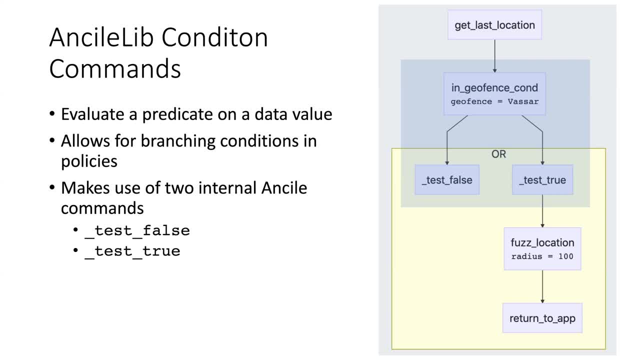 condition commands and style allows for conditions in policy and we do it via these condition commands and how these commands work. they evaluate a predicate based on a data value. so for this example kind of highlighted in in our diagram, the ng offender cond that's going to evaluate the location coordinates that were fetched from get last. 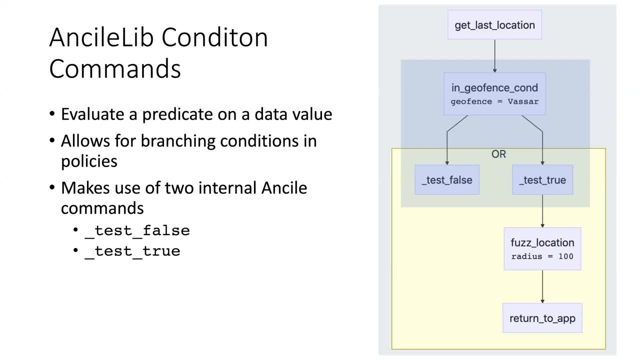 location and it's going to evaluate to see if those location coordinates are inside a vassar or not. What it's going to do is these condition commands. it's then going to advance the policy by executing one of two internal ANSILE commands, and those are shown there as underscore, test, false and 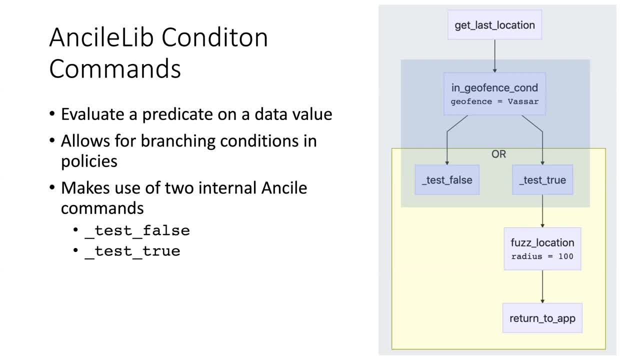 underscore test two And they'll execute one of those depending on the value of the evaluated predicate. So for this policy, if I'm in the geofence test, true will automatically get executed. so those commands aren't called directly And for this policy I didn't need to explicitly specify the underscore test. false condition. 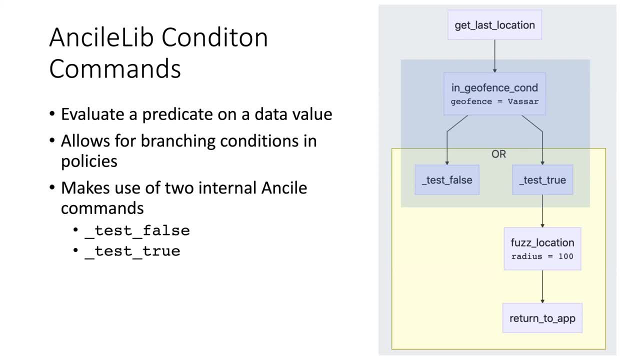 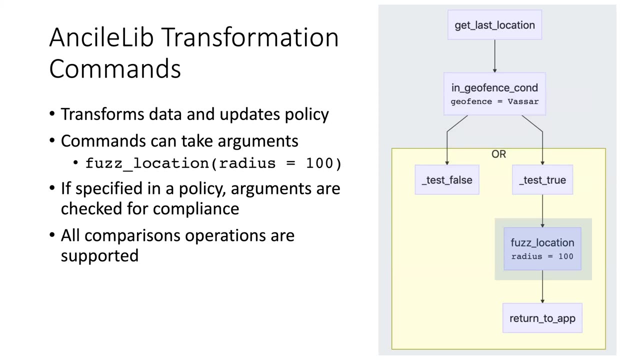 since there's nothing that's going to be authorized If the user is outside of the geofence. but I added it just so you can, kind of you can, clearly see the branching for this policy. So the next type of command are transformation commands, and their purpose is to derive the 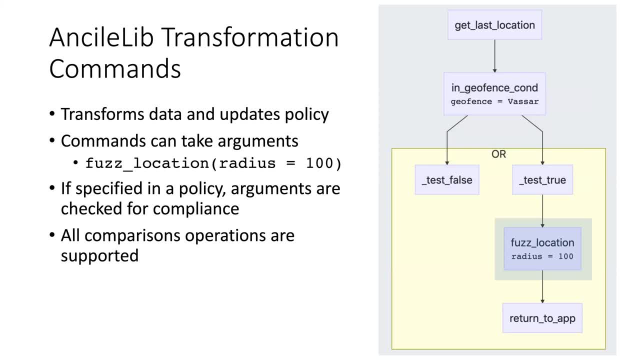 construct derived data and updates the policy. And these commands can take arguments. As you can see, the fuzz location which injects some noise into my location that takes a radius, so kind of how much noise to inject And if an argument, if arguments are specified in a policy, they're going to be checked by. 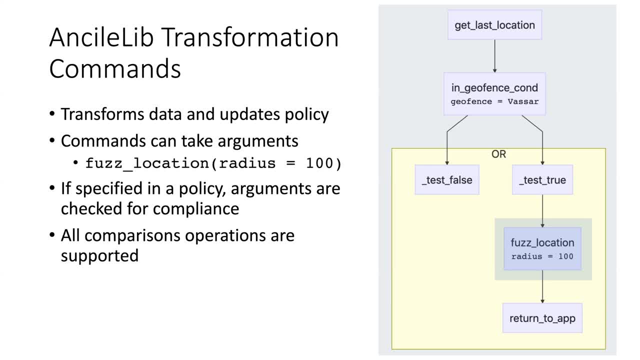 our runtime monitor And so you can see how that's important because the fuzz location function if we didn't check, if we didn't check the parameters, So if we didn't check the parameter, like the radius, that was being passed in a program. 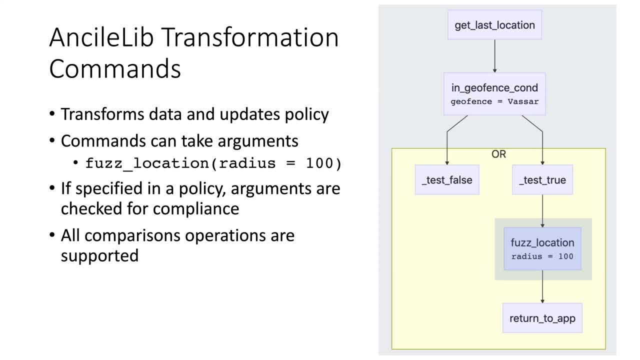 could call fuzz location with a really small radius, And you know the user's privacy if it's. you know, for example, if you called it, the radius of zero wouldn't inject any noise and which would defeat the purpose of having. 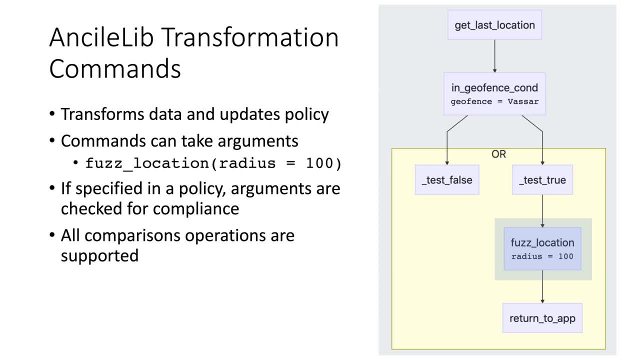 the fuzz location function in there. So if an argument is specified in a policy, ANSI will check that and we can, in addition to doing kind of just e-mailing. We support all the regular comparison operations like greater than less than so on, and so 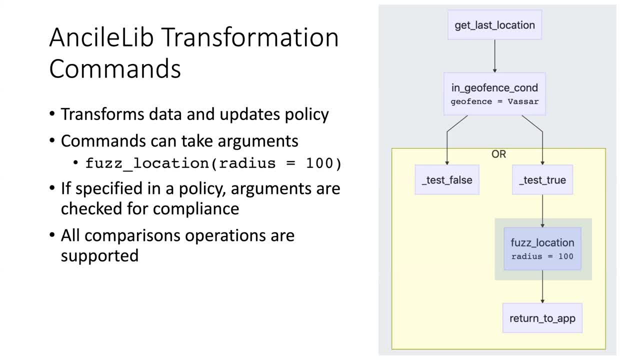 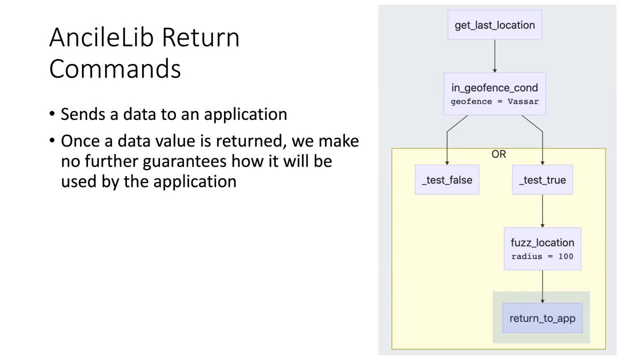 forth. Okay, And the last type of command that ANSI supports are return commands, which simply send data back to the application, And so, for our example, the return to app- that command will return our fuzz location to the application. All right, so that kind of talks about the different types of commands that we support. 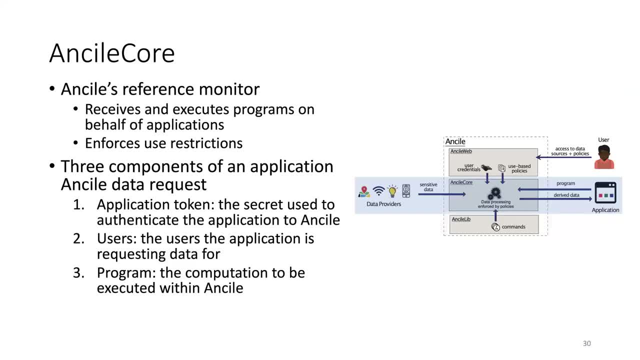 in ANSI-L lib And so the major, the last piece in the major module of ANSI-L is ANSI-L core, And this is our runtime reference monitor, and this ANSI-L core is responsible for enforcing the use restrictions on all of these privileged commands, on these user-submitted programs. 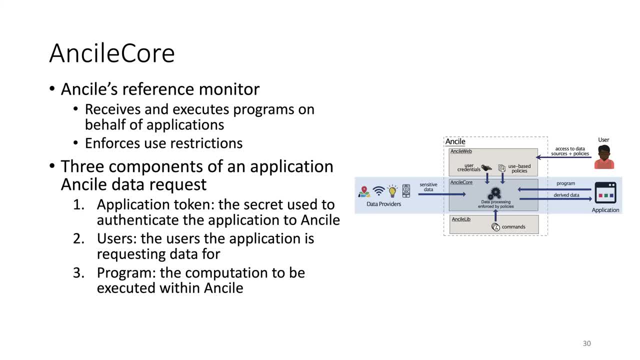 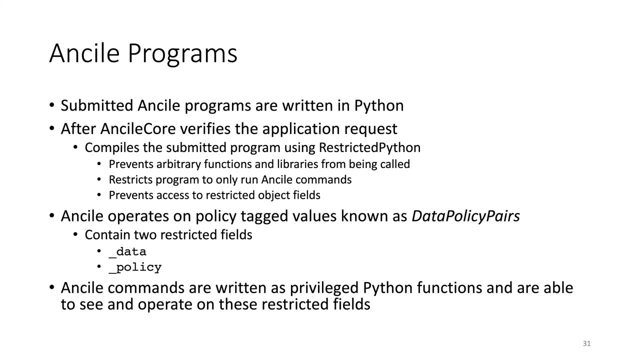 Okay, So in addition to being the runtime monitor, it also handles handling ANSI-L requests, which we previously talked about. So let's talk about kind of the structure of what an ANSI-L program looks like. Programs are submitted by the application. They're written in Python and so after ANSI-L verifies the application, request it then 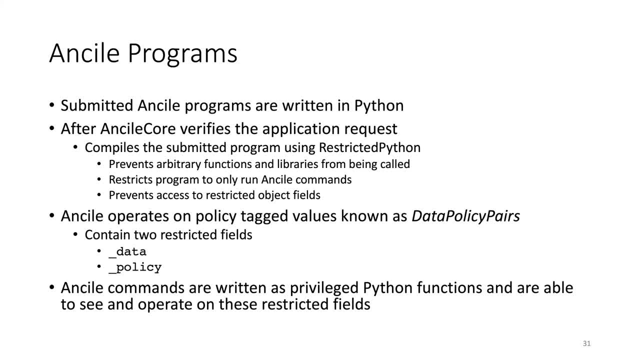 and as part of the request. the request has the program. ANSI-L core will compile the program, and it does that using restricted Python, And this is important because restricted Python prevents arbitrary functions and libraries from being called, And so, in essence, what we've done is we've restricted programming so they can use kind. 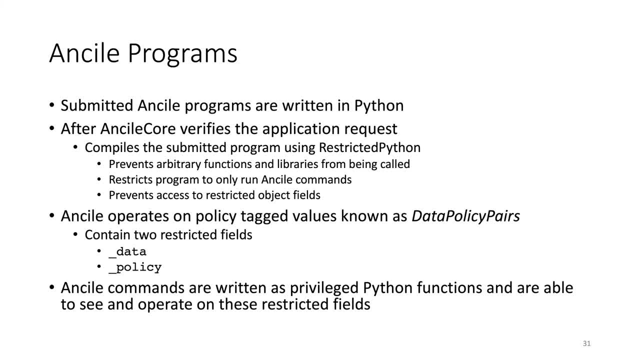 of all the logic and syntax of Python, as opposed to just writing a specific ANSI-L program. Okay, So we've restricted Python to a specific ANSI-L language, but the restricted Python it prevents, it restricts us to basically just running only ANSI-L commands. 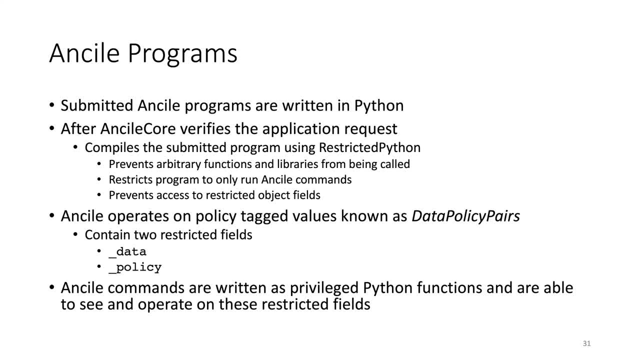 And we use function decorators to make sure that these ANSI-L commands are checked for policy compliance. The other thing that restricted Python does is it prevents access to any restricted object fields, And so, for Python, any field name that starts with an underscore- excuse me- is restricted. 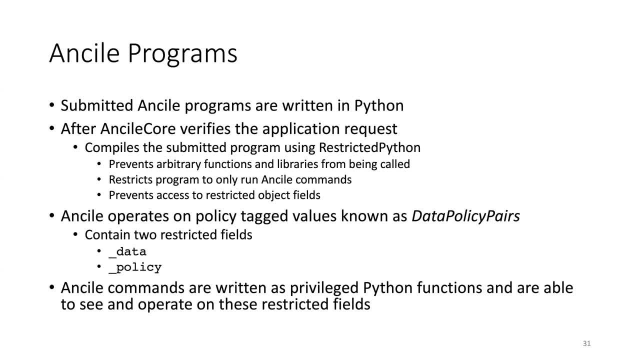 And we use this feature on our data policy pair. These data policy pairs have two fields, two restricted fields. One is the actual data right- You can see how we want to hide that behind privileged commands- And it also has the underlying policy associated with that. 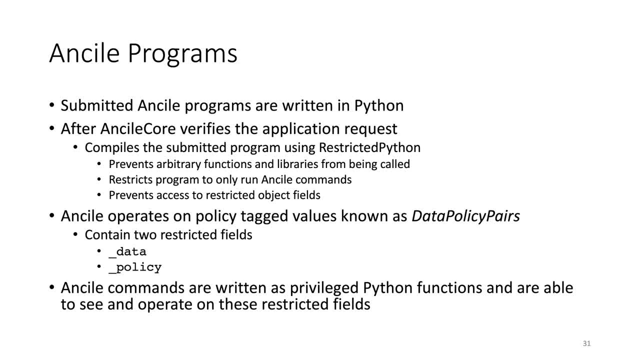 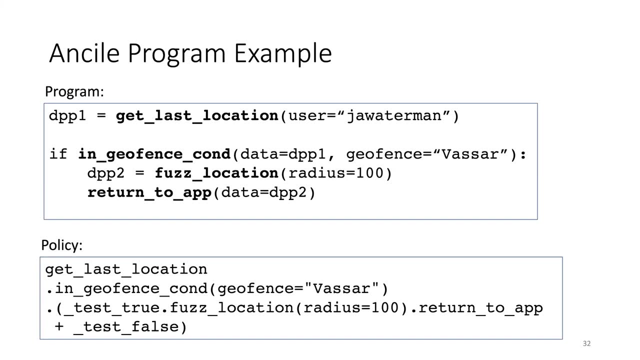 So those fields can only be accessed inside, And not by the program itself, but only when they call these restricted commands which we check for policy compliance. All right, Let's take a look at a program example of the program that we, the scenario that we. 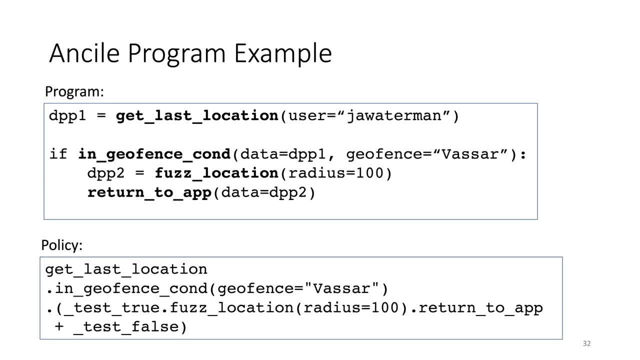 are running example that I've described, And so down, at the bottom shows our policy, And on the top we have our policy, Okay, And then we have our program. So get last location. That's going to fetch my location And again, that's one of these external commands that get data source. 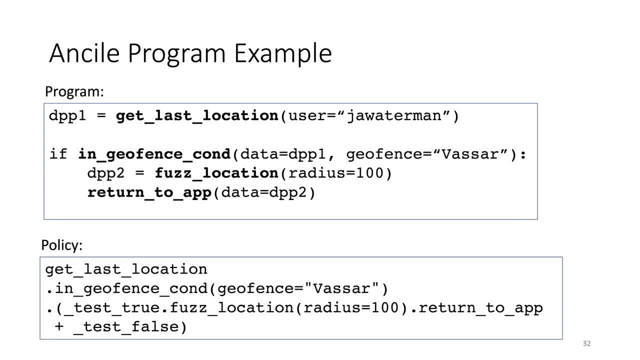 And so that's going to return a new data policy pair which I've assigned as DPP data policy pair one. Okay, And so that's our data policy pair, And as far as the program's concerned, that's really treated as kind of an opaque. 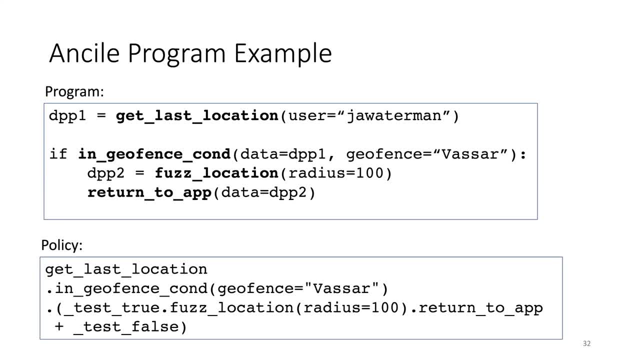 And again, this is our data coupled with our tag policy. but in the program itself, really, we can just kind of pass that around. We can't inspect the data, We can't inspect any of the policies associated with that, but we can call these ANSILE commands. 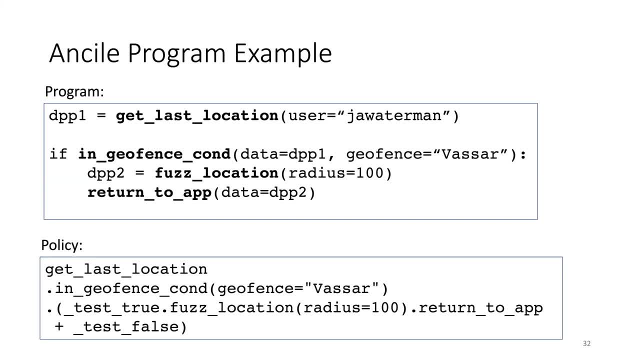 And so the command in geofence condition, that's a condition command and we pass in to our arguments, We pass in our data policy pair and we pass in an argument letting us know what geofence is, And so this is a condition. since this is a condition command, it actually doesn't create. 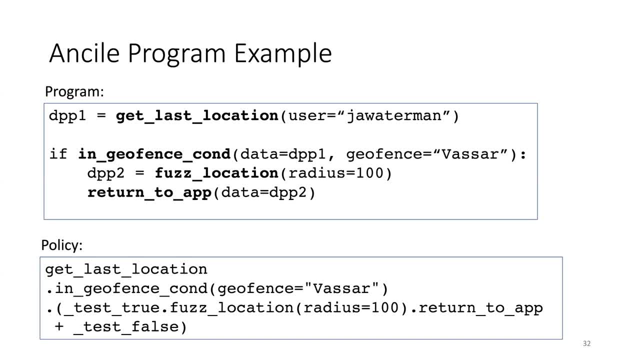 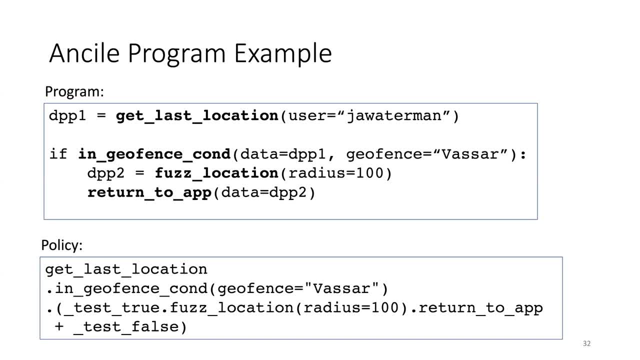 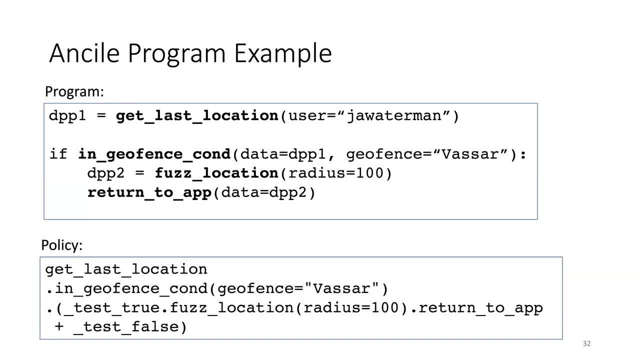 part of the contract is that they can return the value of their predicate. So that means we can use these commands in like a if statement, as we have here, And so if we are in fact inside the geofence, We can then fuzz our location. and this fuzz location, this is a transformation command. 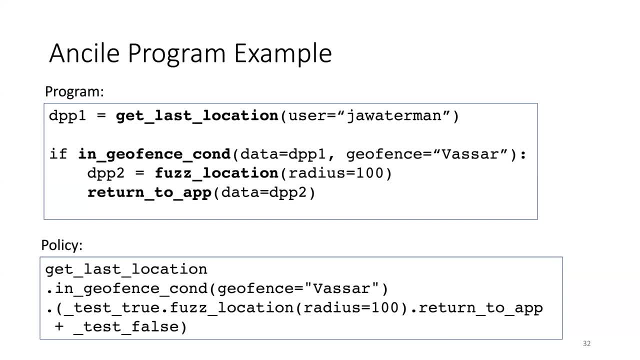 And since it's a transformation command, it's creating a derived value, and that derived value is going to have a new data policy pair associated with it, which I've assigned the variable DPP2.. And so that's going to be the fuzz location and the corresponding updated policy for that. 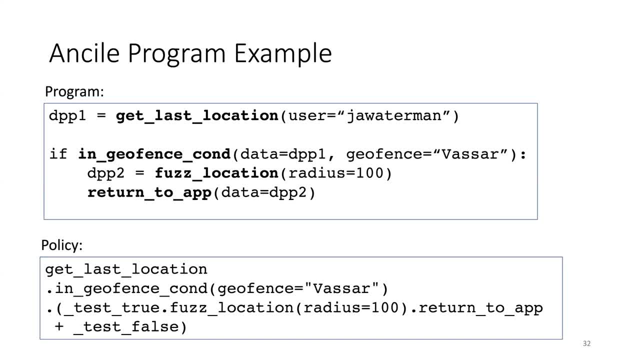 And you can see. then the last command is the return command: return to app. and here we're passing in data policy pair two. So note, if we return to app, if we passed in not data policy pair two, the one that has been fuzzed, if we passed in data policy pair one, that would fail. 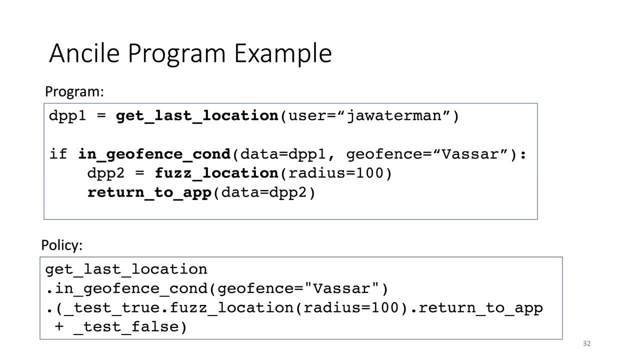 Our runtime monitor will catch that, because at that point data policy pair one: well, the location hasn't been fuzzed yet, so its policy would not be authorized. It would be authorized to return to the application because that location hadn't been fuzzed from. 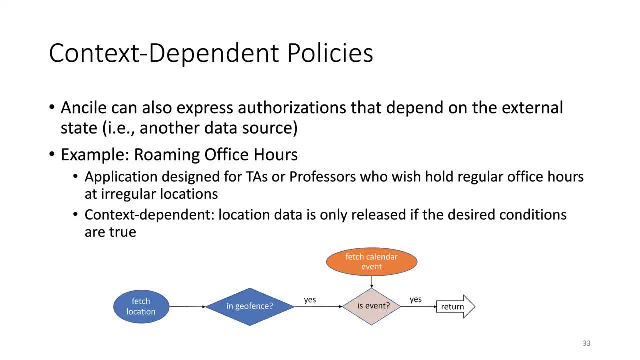 there, Okay. So that's kind of a straightforward example. but ANSI also supports authorizations that can depend on external states of another data source. So, for example, let's say we have this idea of roaming office hours, Where a professor would like to hold office hours at scheduled times. 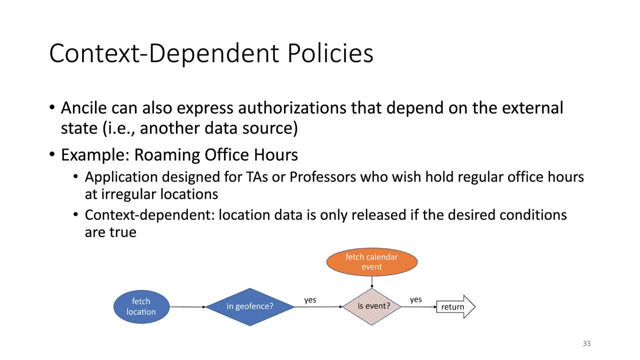 So they posted from two to four. on Tuesdays I'll be around, but these office hours might be held at irregular locations, And so you might want to have a policy that you will share your location first of all if you're on campus. 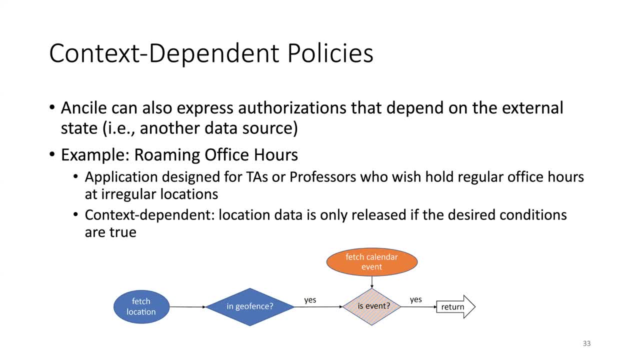 So if you're not on campus and even though you're holding office hours, if there was an emergency or something like that- you don't want to share your location. So you want to share your location only if you're on campus and only when your calendar. 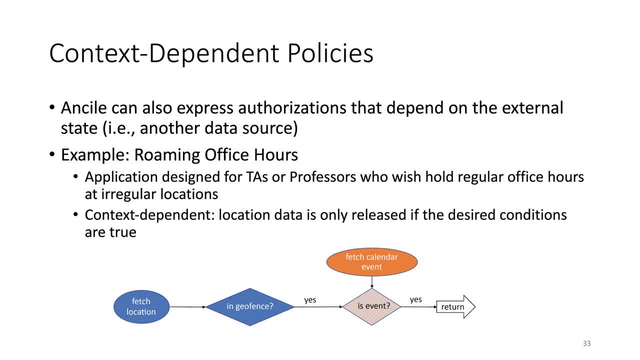 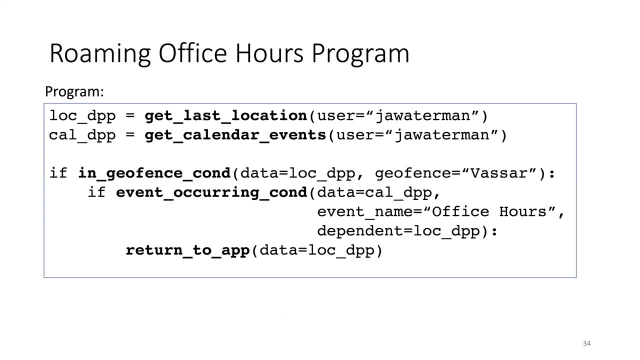 says you're holding office hours, okay, And that's kind of demonstrated by the diagram down at the bottom, And the program for that is here. And so notice how we have two data sources now. We have a location data source and we have a calendar. 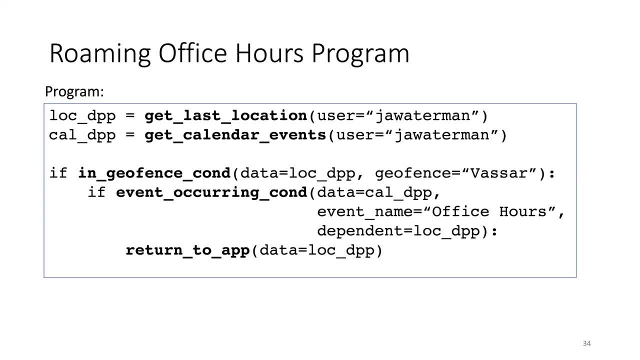 So we're going to get- we're going to have two external commands: get last location, as we saw before, we'll return as a location data policy pair and then we also have get calendar events And that's going to be our data policy pair for calendars. okay, 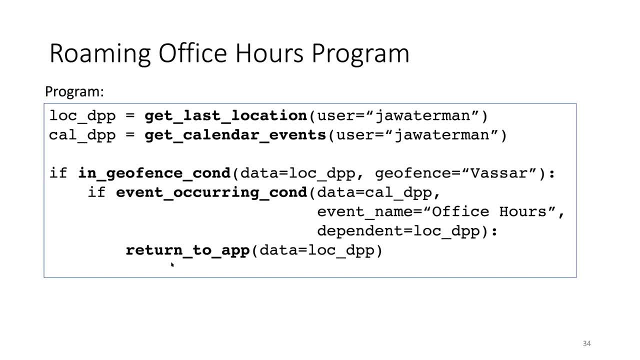 And so what we've done before. first, what we want to do: just like in the previous example, we want to check to make sure that we're on campus. So we're going to use this In geofence condition, just like we did before. 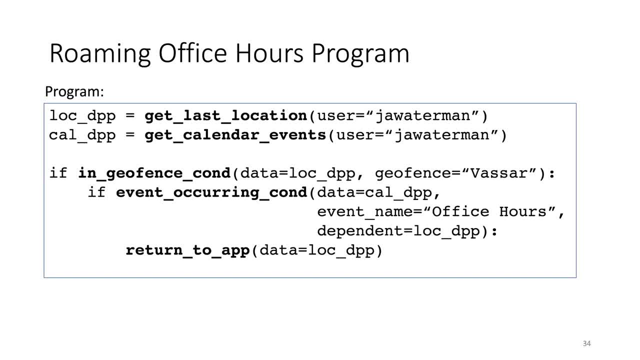 And that will advance the policy, whether it's true or false. And then if we are in fact in the geofence, then we can call this event, this event, occurring condition, okay, And what's different about that? so we're passing in the calendar data policy pair and we're 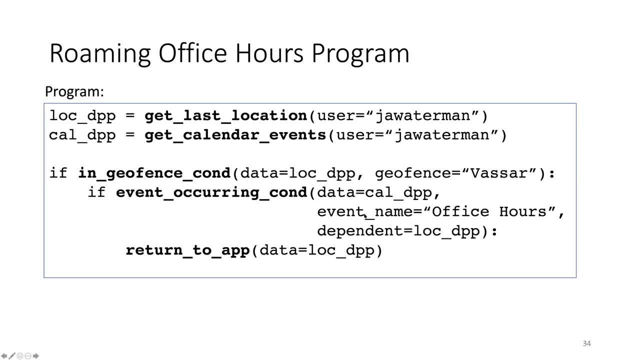 looking for the event, The calendar event that we're looking at, And but what we've also passed in is this argument, this dependent argument, which is our location data policy pair. okay, And what that means is is that this dependent policy makes sure that it's going to check. 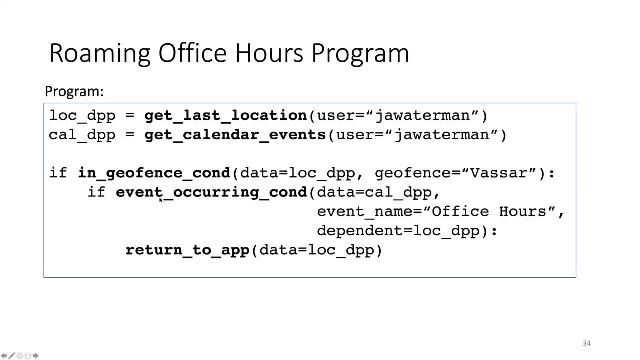 both the calendar and the location to make sure that both of these policies are going to be authorized for and compliant for that. okay, So both of those are going to be checked To make sure that they're in policy compliance And then, finally, if this condition is true, then we can return the location, right? 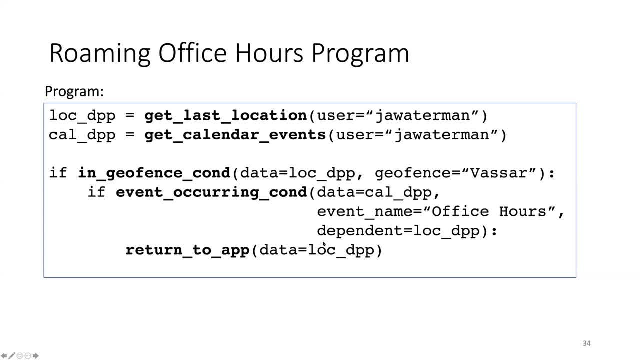 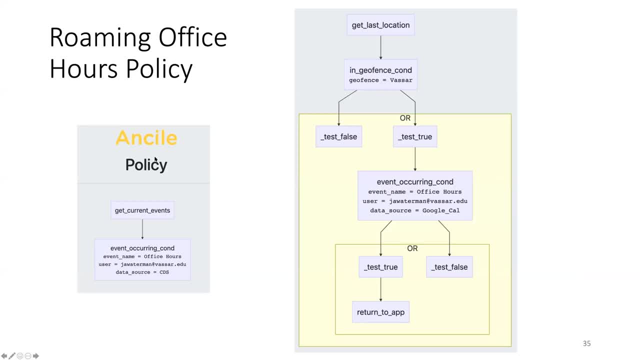 We don't have to fuzz it or anything like that, because that wasn't part of the policy from there. Okay, And so if we take a look at what those policies look like- the policy for the calendar shown on the left- and it's a very simple policy, so we allow it to get the current events- 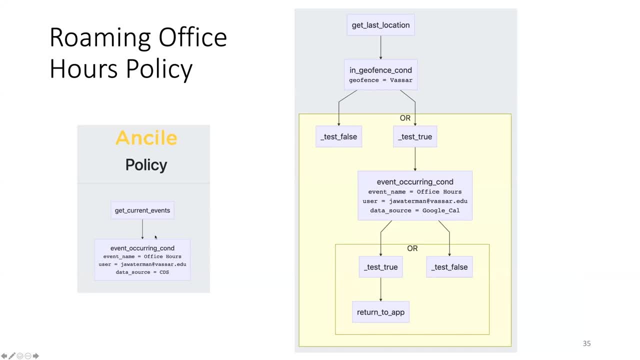 and we're only going to authorize: Okay. So if we have this occurring condition and we match our office hours, okay, And we also show that the dependent data source is our location services. CDS is our campus location service. from there and on the right, we have our policy for our location. 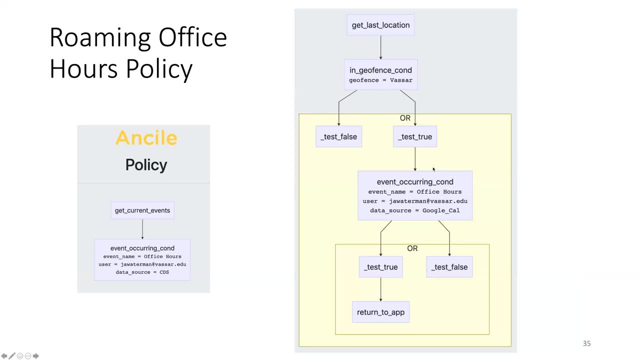 And again, we have our test to see if we're in the geofence, and if we're true, then we'll call this a current, this dependent condition, and if that is in fact true, then we'll return to app. 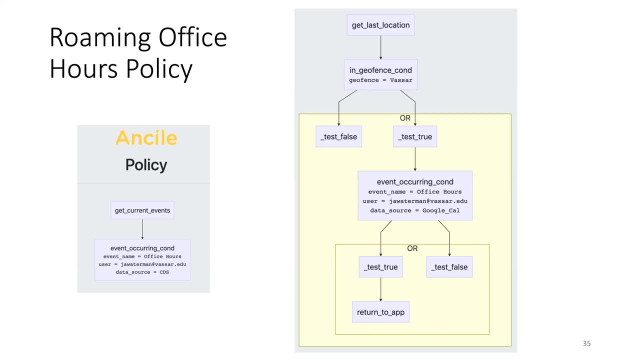 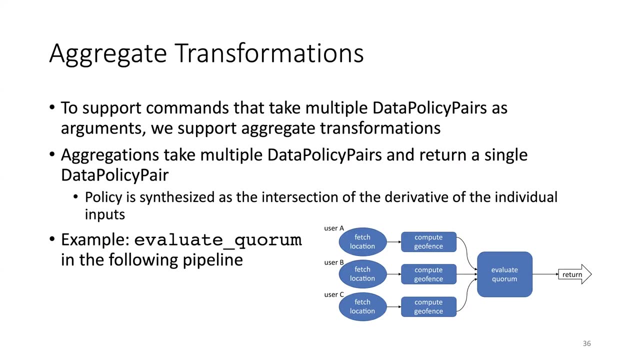 Otherwise, we're not going to authorize the application to return anything. Another feature that ANSILE supports are aggregate transformations, So these are commands that take multiple data policy pairs as arguments. We call these transformation aggregations. Okay, Okay. So what we're going to do is we're going to take multiple arguments, because they take 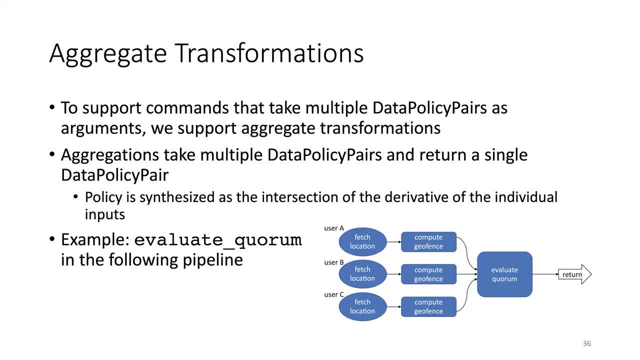 multiple arguments and they return a single data policy pair with a new policy associated with it. This new policy is synthesized as the intersection, as the derivative of the individual data policy input data policy pairs, And so in the diagram to the right, which I'll go over in more detail on the next slide, 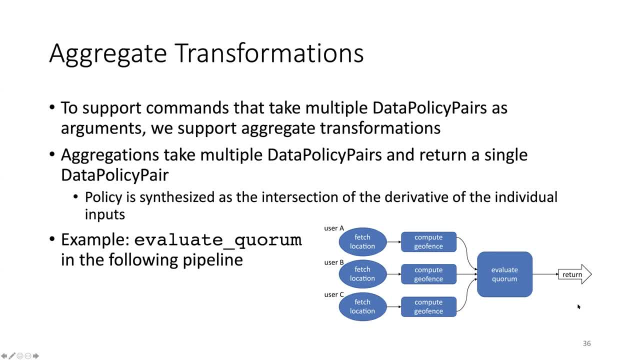 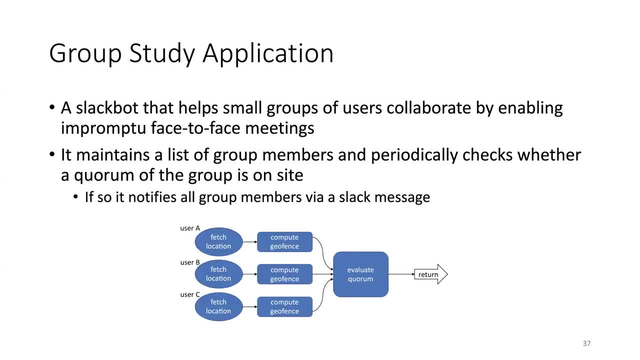 the evaluate quorum transformation is an aggregation. It's taking data policy pairs from several users. So to show off our aggregation feature and to show support for aggregation transformations, we created a group study Slack bot. So this is a Slack application and you can basically create a study channel and this 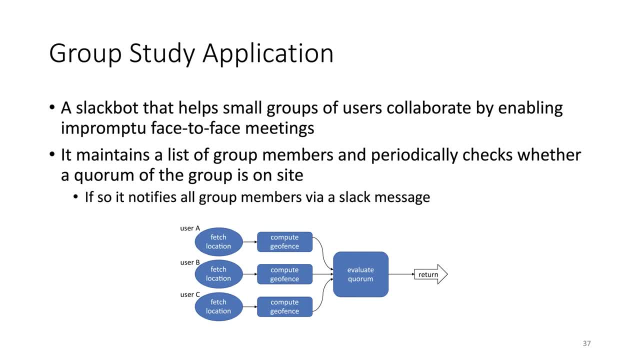 is going to help us facilitate meetings with small groups of people. By the way, this is a Slack application. So this is a Slack application And you can basically create a study channel, And this is going to help us facilitate meetings with small groups of people by using the group. 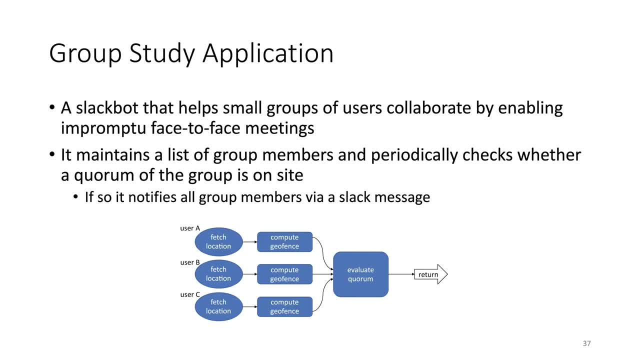 by enabling impromptu face-to-face meetings. So with a Slack bot you can create a channel. You can sign up via the Slack bot interfaces with ANSI also. You can basically authorize to share your location. And what the Slack bot does is it periodically checks your location and it sees whether 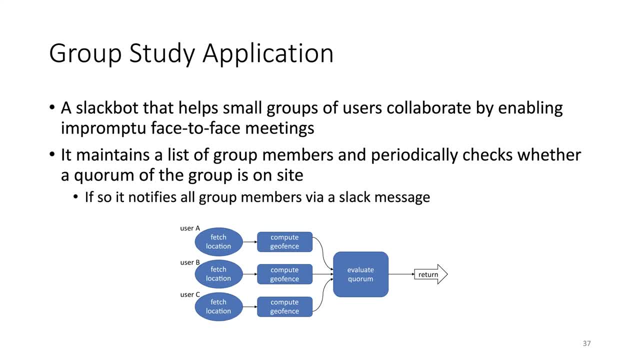 a quorum of the group is on site on a specified geofence, say like the library, And so if you're all meeting at the library, Then it simply messages the group on their Slack channel that hey, everyone is here. 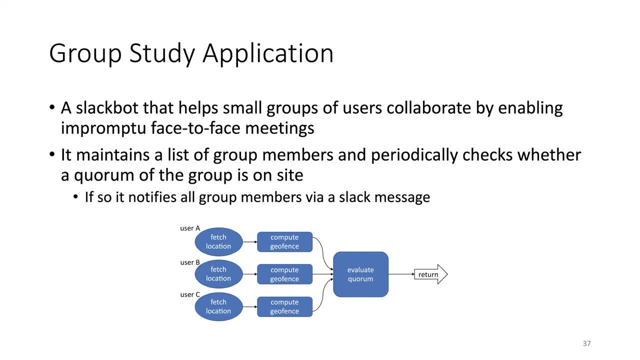 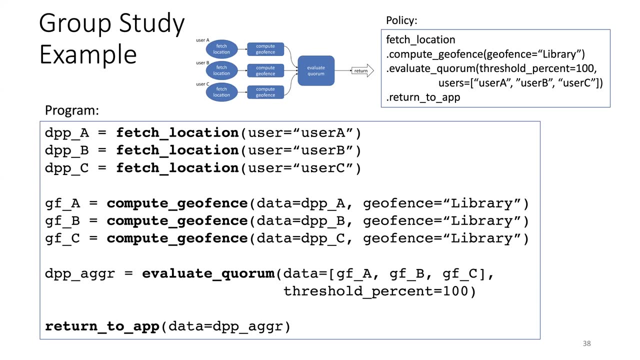 You should maybe you know, if you want to have a meeting go, you know you're allowed to, But it doesn't share. it doesn't share any of the individual user locations, And so here's the associated so kind of the. it's a busy slide, but there's kind of the. 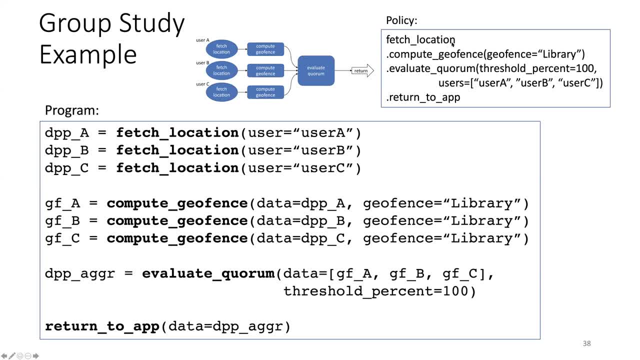 pipeline diagram, The particular policy, Which again is, I don't know, I don't know, I don't know if you've seen this, but is so all the users would have the same policy, or could have They get a difference? 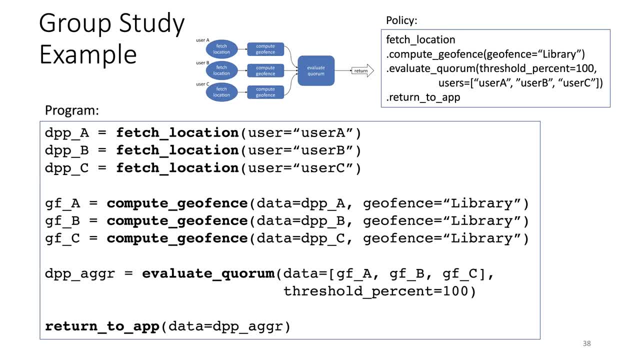 But for this example all the users have the same policy, which is allowed to fetch location and then compute the geofence on that location, And so notice here in this case, right. the previous example was using the condition command to return a condition, whether you're in the geofence or not. 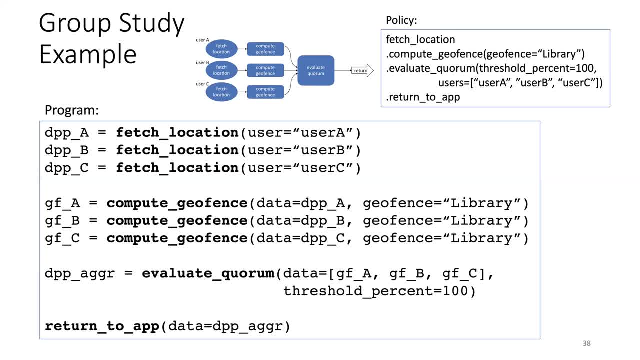 But in this case we don't want the condition. We actually want the Boolean, whether we're in a geofence or not, because what we're going to need is we're going to have an aggregation function, this evaluate quorum, which is going. 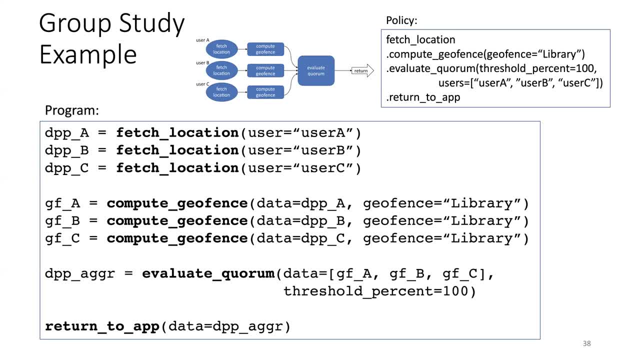 to take input from all of the users- all of the users, whether they're in the geofence or not- and then compute whether there's a quorum, whether everyone is there. And so, for this program example, I've set the threshold percentage to 100, which means 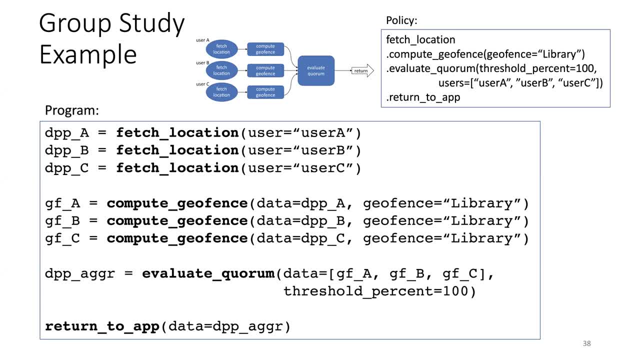 everyone needs to be in the group for us to get notified, And so, if we look at the program, So we have three users- Users A, B and C- And then we have the user A, B and C here for this. 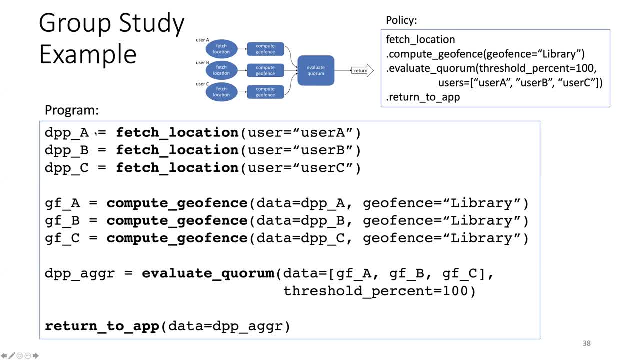 And we're creating the three data policy pairs A, B and C for that, And we're going to compute the geofence for those individually. And so here this is an actual transformation function, It's not a condition command. 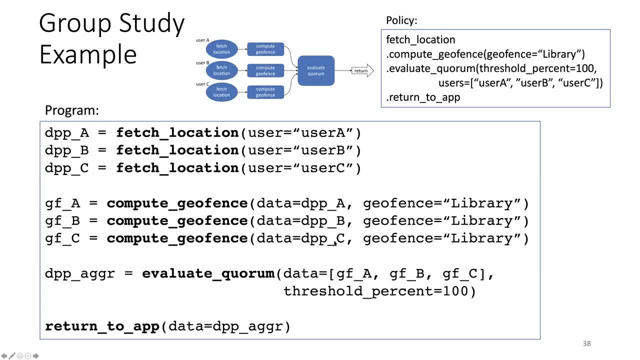 It's a transformation, So it's taking the respective data policy pairs as input And it's returning a new geofenced data policy pair, right, So this, you know, the data, this derived data on here is just going to be a Boolean. 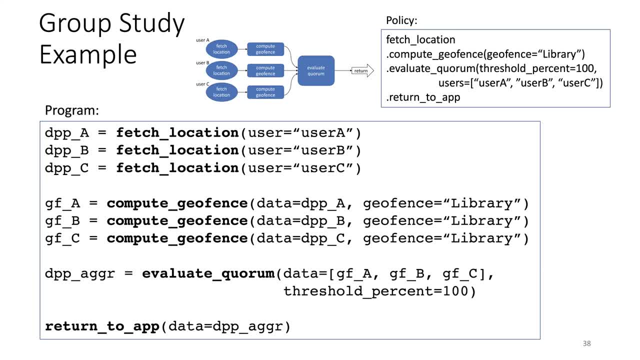 whether you're in the geofence or not, And then the correspondingly advanced policy. with that, okay, And so the evaluate quorum, our aggregation. this now takes a list of data policy pairs and the threshold percentage, And again, this is also a transformation. 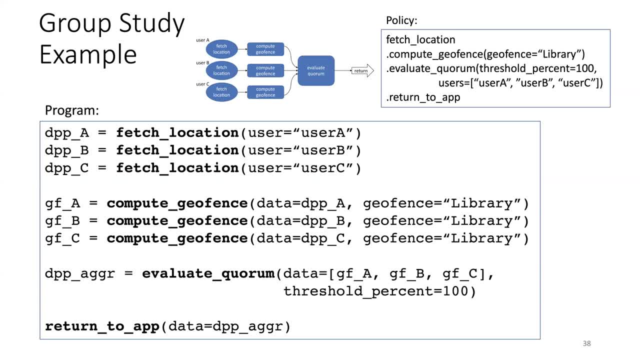 So it's going to return a new data policy pair which is just whether this is whether there's a quorum present. So no longer That data policy pair, No longer It's going to return the individual Booleans whether who's there or not. 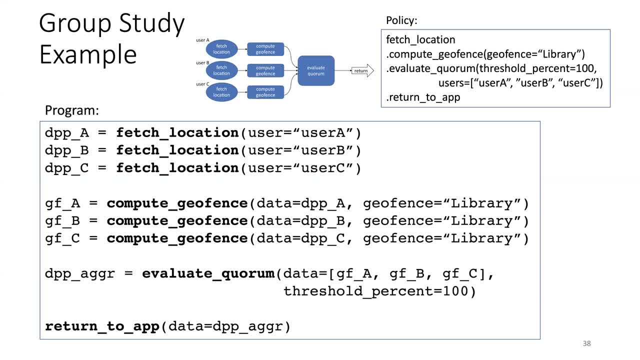 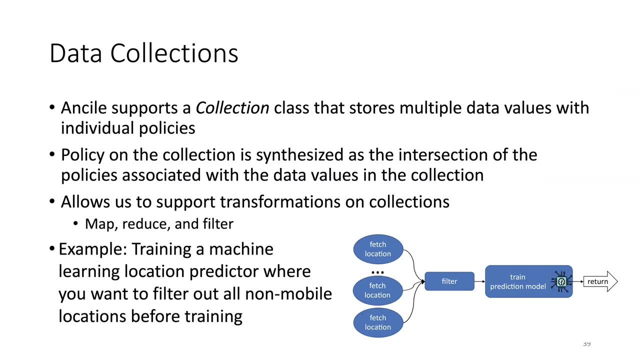 It's simply the aggregation of all of those, And then what is actually returned to the app is just simply whether everyone is there or not from there. okay, So no user's location is leaked to Slack. It all stays inside of ANSILE. 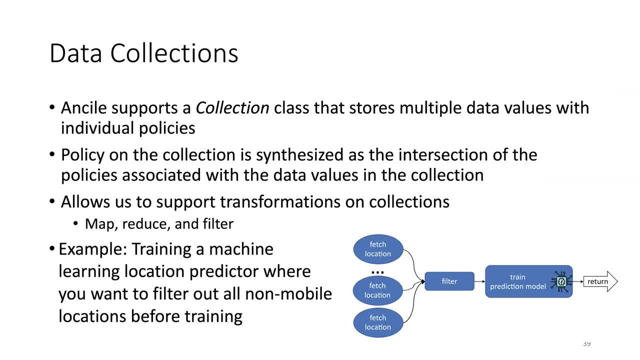 The last feature in ANSILE that I'd like to talk about is ANSILE support for collections. So collections are a class that stores. It stores multiple data, data values And what's different from the aggregation each of these individual? we keep each of. 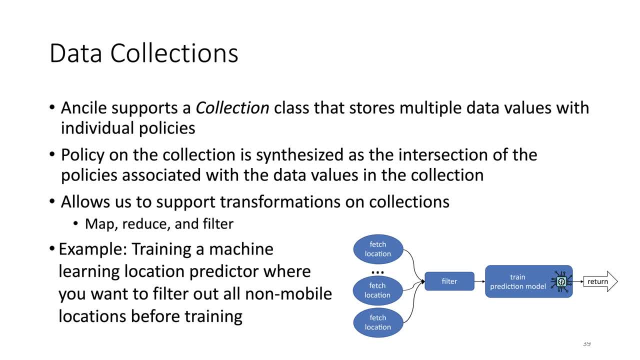 the individual policies intact. right, As we saw from the last example, the aggregation function. it returns a new data policy pair that moves the that has its own associated policy with it And it kind of loses the history. So collections allow us to keep the individual. 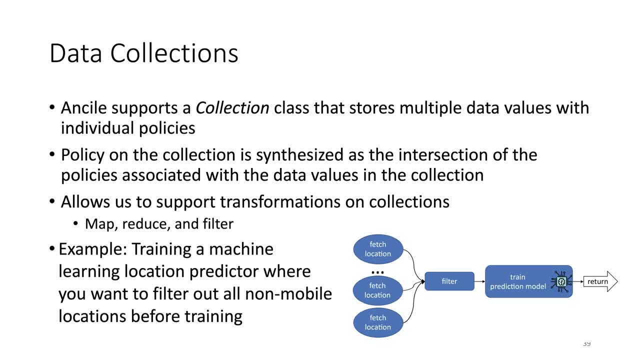 Individual: Yeah, Individual policies intact. okay. So, even though we have the individual policies, the policy on the collection, the policies, the collections do have policies and they're generated. they're synthesized as an intersection of the policies associated with the data values on the collection. okay. 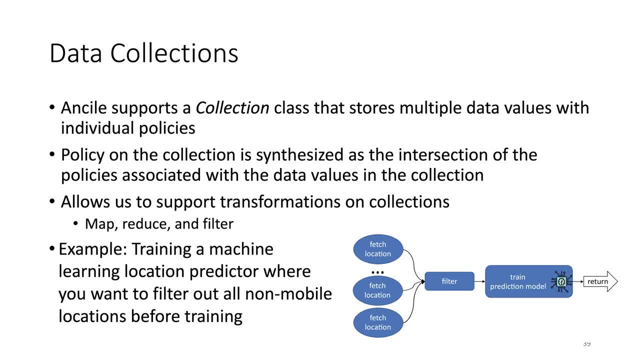 So this allows us to support, easily support transformations on collections, such as map reduce filter. So, for example, to show off collections, we built a machine learning location predictor which basically takes a history of user locations and then predicts right. 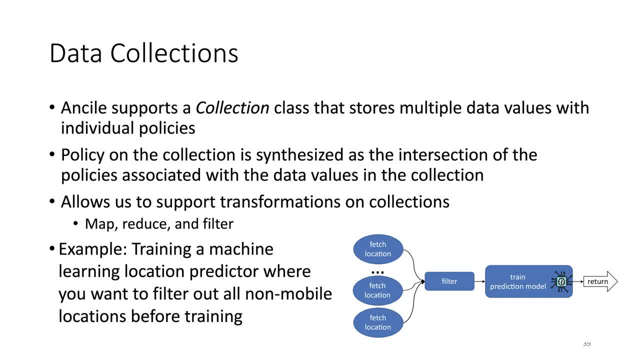 This would be good for intelligent spaces, where you can build models of of when we, should you know, turn down the heating or turn off the lights and things like that, And so, for this example, the location values were stored as a collection, and storing them. 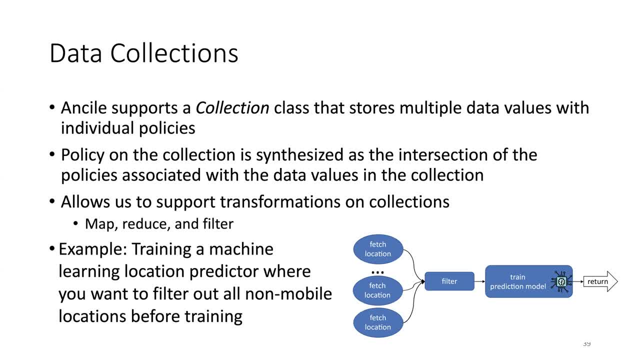 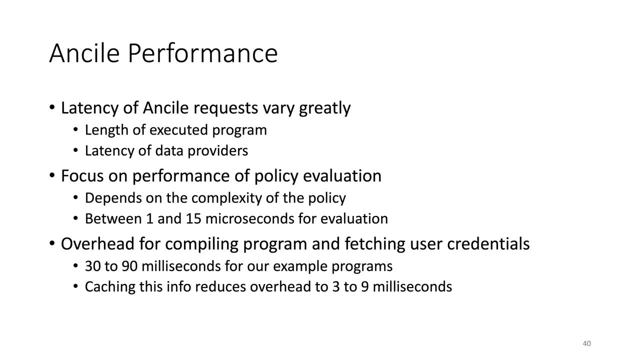 as a collection, made it easy to filter out all the location data from non-smartphone location sources From there. Okay, So that's kind of the tour of the main features of ANSILE and we kind of looked at some examples. 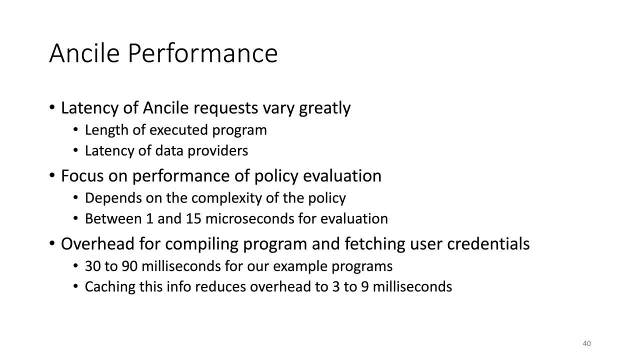 And so you know, we built these kinds of prototype applications and then we took a look and tried to, you know, characterize ANSILE's performance And it turns out right. so you know, a request actually has a lot of components, and these 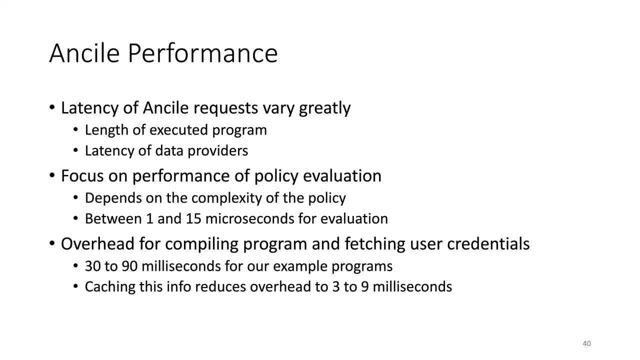 requests can vary greatly. They can vary based on the length of the execution. So how many commands like, for example, the ML program right, training up an ML model? that command takes certainly a lot longer than calculating a geofence right. 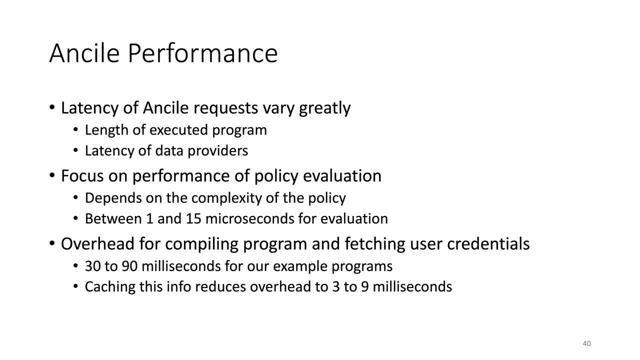 So the latency of these requests vary depending on the what commands we're executing in the program and the latency of the data providers- Some of them, particularly when we're calculating calendar. there's a lot of variance from them And so, in a sense, right, we don't really have a lot of control over that, right. 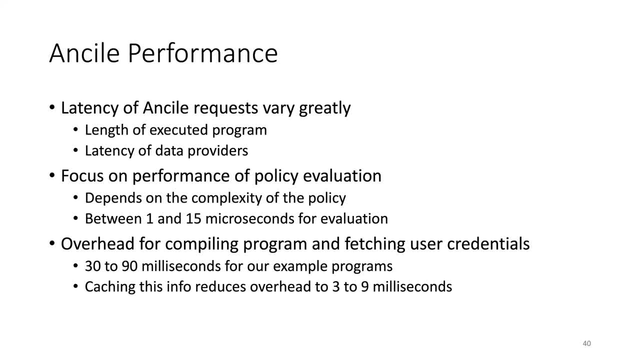 So what we did was for performance. we focused on the performance of policy evaluation And you know, not surprisingly, how long it took to evaluate the policy. depended on the complexity of the policy, But for all of our prototype applications, evaluation took between 1 and 15 microseconds. 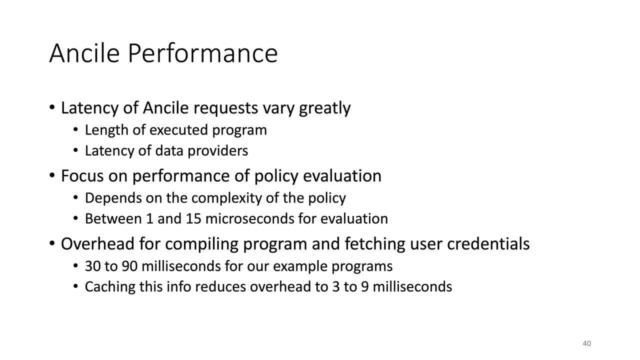 So not a substantial amount of overhead From there. The other thing we looked at is the overhead for compiling a program, right? So when a request comes in, the first thing that we do is we take that program, which is just, you know, a source Python program, and we need to compile that. 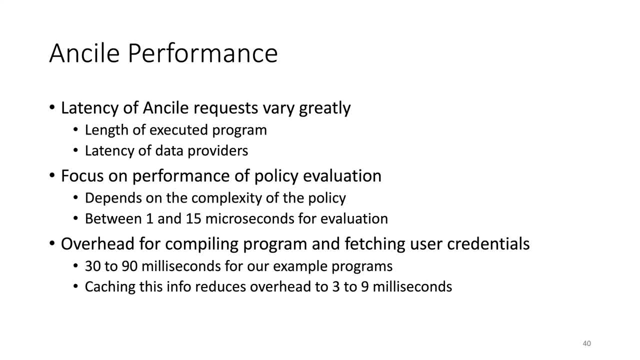 We need to compile that under restricted Python and fetch any associated user credentials, And so, as you imagine, that takes a little bit more time. For our example, programs that took anywhere between 30 and 90 milliseconds, And we saw that that could be a bottleneck. 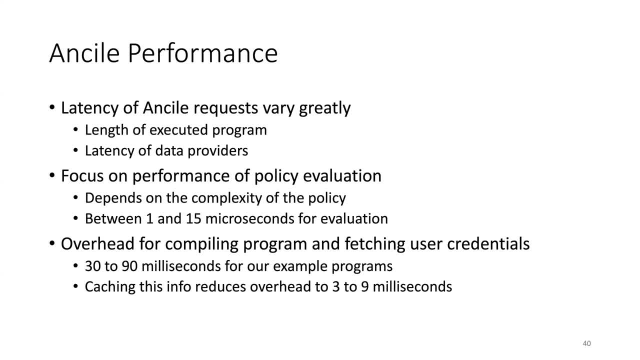 So what we did was we implemented caching in our system, And so the first time a request comes in right, we have to compile the program. There's no getting around that. But we'll cache that compiled program around for a while. 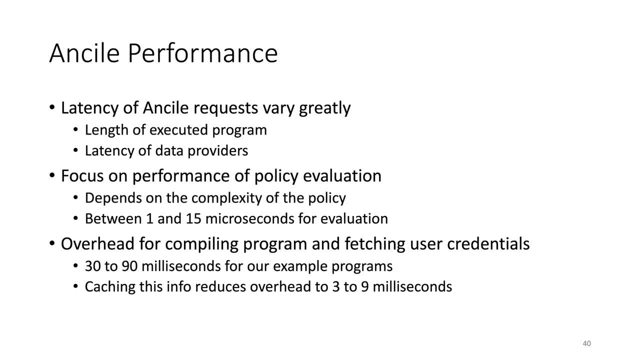 And so, if that request comes in, again with the same program and the same user. so think about our Slack bot, right, It's pulling, you know, every like minute or so It's sending the same program with the same users. 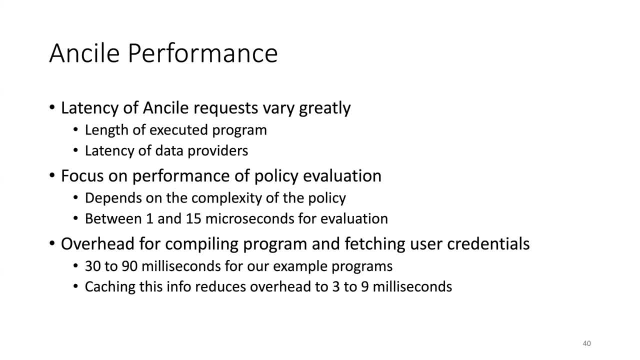 So, And so we cached that, We cached the program, We cached those requests And that reduced the overhead by an order of magnitude. right, It went from about 30 to 90, down to 3 to 9 milliseconds. 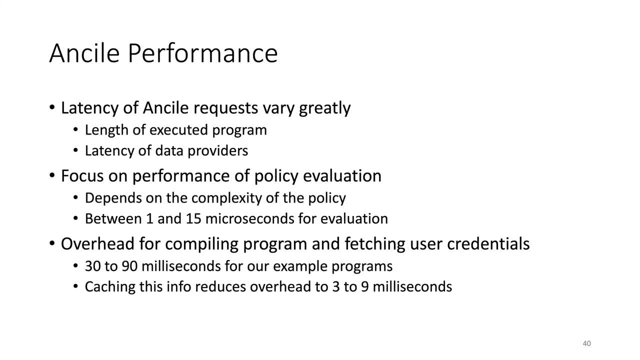 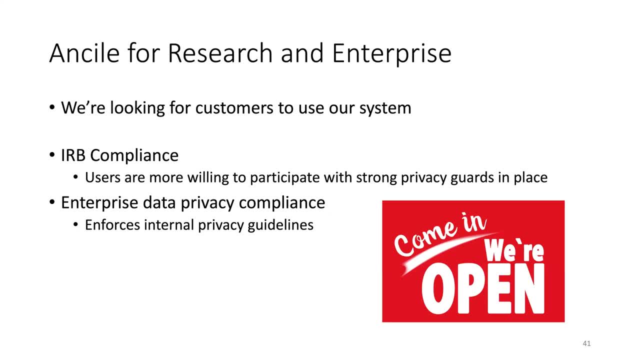 So that, I think, was, you know, a good win there, And so we developed this system, kind of you know, and we're really looking for customers now And so if you're, you know, if you're interested in kind of thinking about how you could use 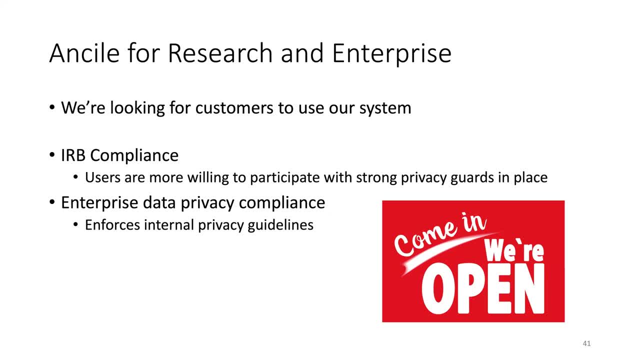 something like ANSILE in your work. please let me know. And two areas where I think you know ANSILE, I think could really kind of you know work very nicely, is with you know IRB compliance right. 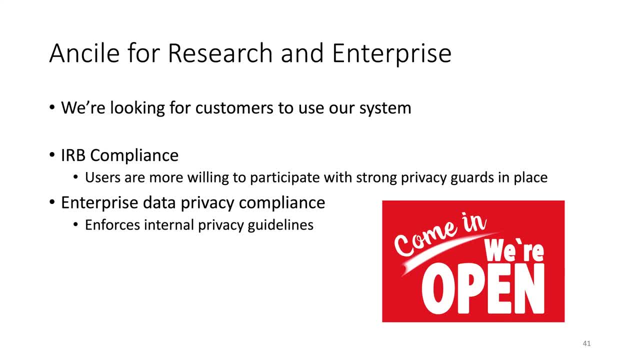 So you know, we have to go through all of these steps to make sure that we're treating data under these restrictions. It'd be nice to actually say, yeah, we've built these policies, these IRB-compliant policies, and we run our- you know, our pipeline, our processing through ANSILE. we can guarantee. 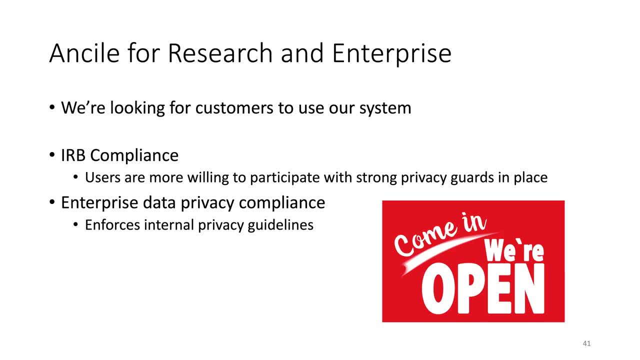 you know, with audit trails and logs to kind of prove that that we are in fact in IRB compliance right. And I would argue that you know, knowing that there's strong safeguards in place, I would think users would be more willing to participate with that. 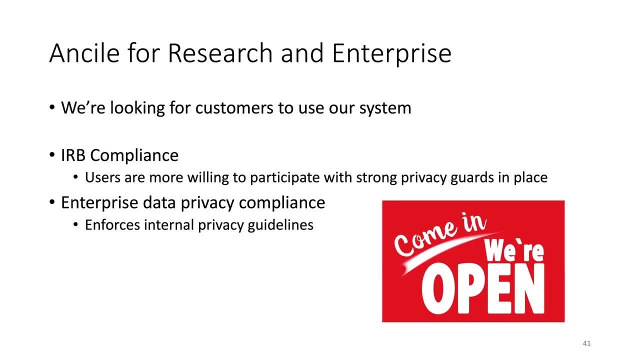 And I think another area where I think you know ANSI will fit very nicely is enterprise, you know, and internal data privacy compliance. We're hearing that, you know, Facebook and Amazon, you know, are kind of coming up with their own internal IRBs. 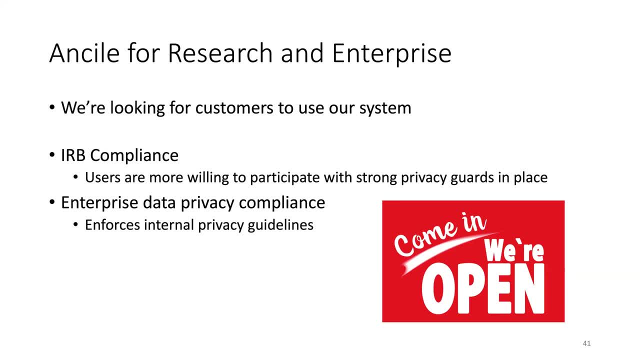 to enforce their internal privacy guidelines. And so here you know, you'd be protecting, not necessarily against someone malicious, but just making sure that they, you know, don't have a bug or somehow don't know the rules and somehow miss using that data. 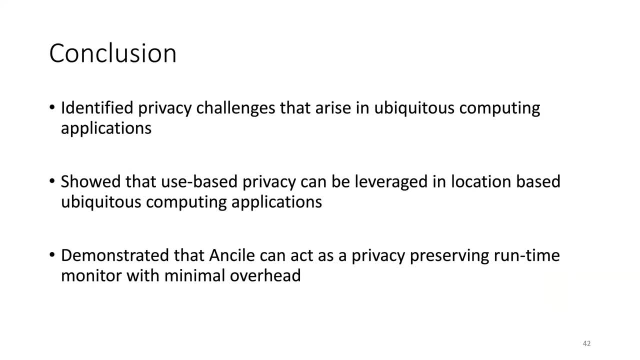 So to kind of wrap up, we talked about some privacy challenges that arise in ubiquitous computing. Hopefully I've demonstrated that use-based privacy can be leveraged and in particular location-based ubiquitous computing outliers, And we've shown that ANSI can kind of meet these privacy needs. 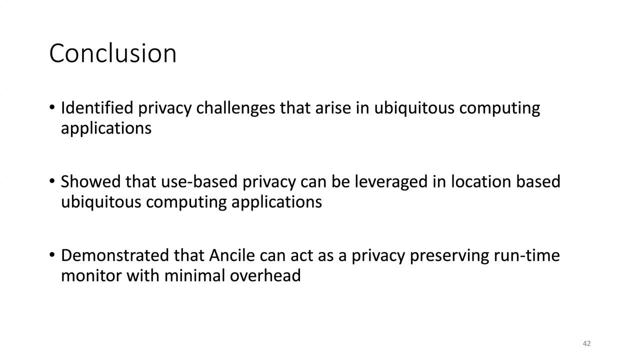 with this runtime monitor and the overhead isn't too bad. So with that, I will stop and take your questions. Great, Thank you. I'm going to just throw up some slides real quick here just to go over some news that's impacting our trusted CI community. 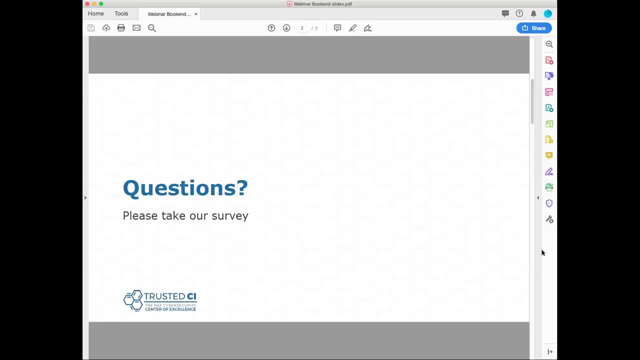 And we'll let some questions pile up and then we'll go through them together, Okay, So first, if you have any questions, please type them in the chat box by clicking on the little chat icon, And also we have a survey that we would like you guys to fill out. 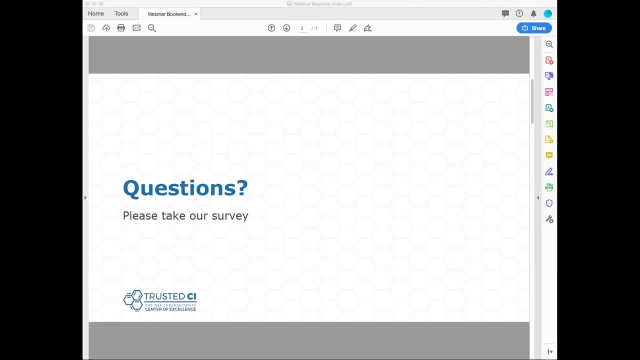 Let me just put this in the chat so that it's a hyperlink that you can actually click on. Here we go. So if you would like to give us a little bit more information, give us some feedback about this presentation, or if you'd like to suggest topics or presenters, go ahead and fill out our survey. 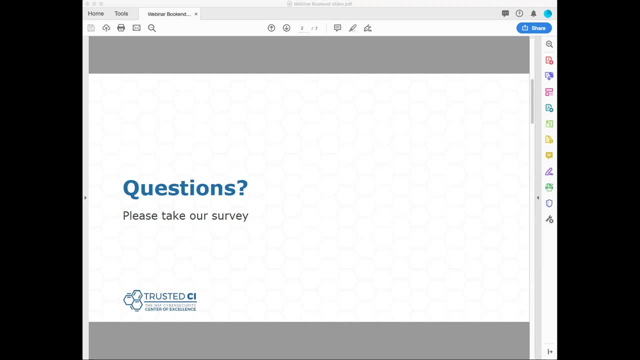 and fill in the comments section with the suggested presentations, And then next up we have a reminder. Trusted CI has a number of things that we're doing at PERC, which is next week, So it's really coming up on us. We've got a workshop. 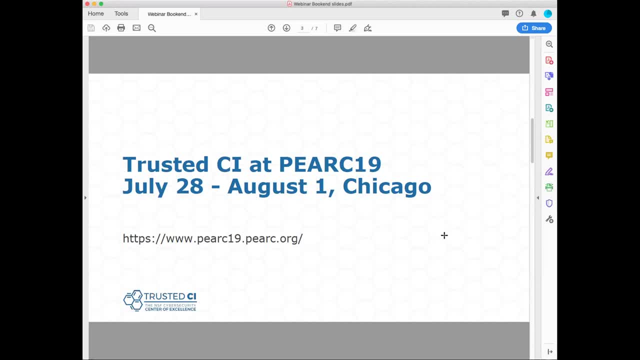 We've got a panel. We're presenting our technical paper. We've got a booth, So if you're going to have a chance to come in and talk to us, we'd love to hear from you. If you're coming to PERC, please come and find us. 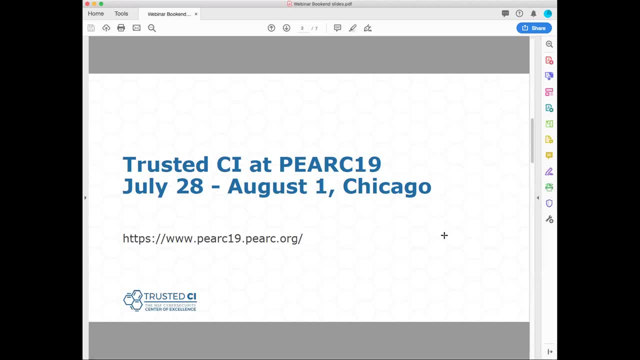 Registration for PERC is closed because they hit their maximum, which is very exciting. So if you are attending, come and find us Say hi. Also. our Cybersecurity Summit, the Trusted CI Cybersecurity Summit, is October 15th through 17th in San Diego. 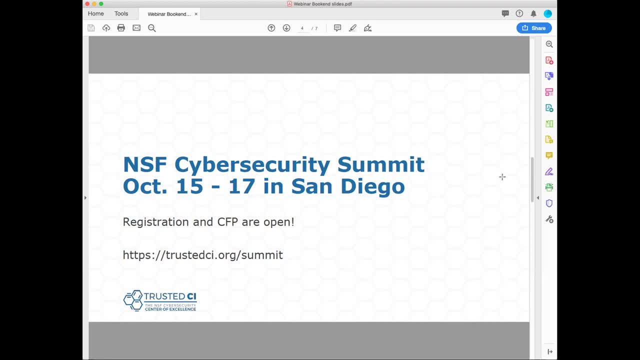 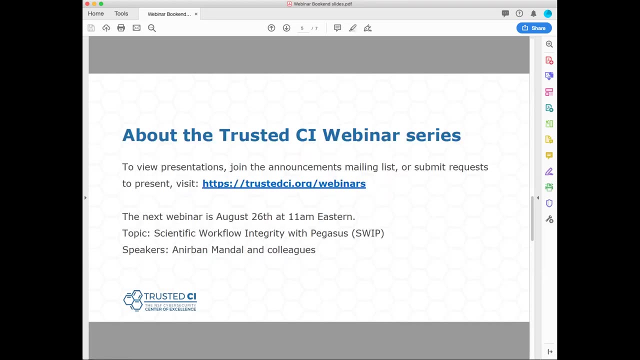 The registration form is open. The call for presentations participation is open. So please check us out at TrustedCIcom. You can find us at TrustedCIorg slash summit and apply or register to attend or present a topic. And then just a little bit more about our Trusted CI webinar series. 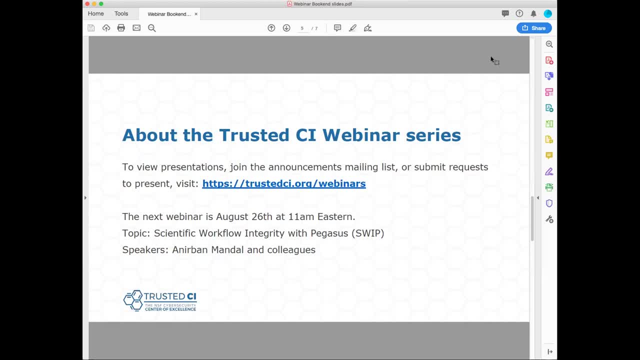 To view presentations. to join the announcements mailing list, submit requests. visit us at TrustedCIorg slash webinars. Our next webinar is August 26th at 11 am Eastern. The topic is the scientific workflow intelligence, And we're going to be talking about the scientific workflow intelligence. 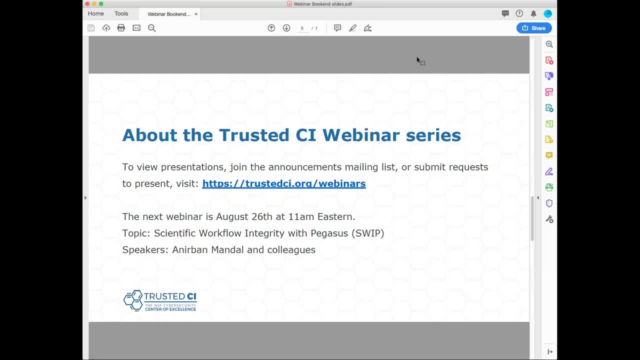 And we're going to be talking about the scientific workflow integrity with Pegasus, also known as SWPPP, And our presenters are Anirban Mandal and his colleagues. So with that, let's go through a question. here We've got Jason. 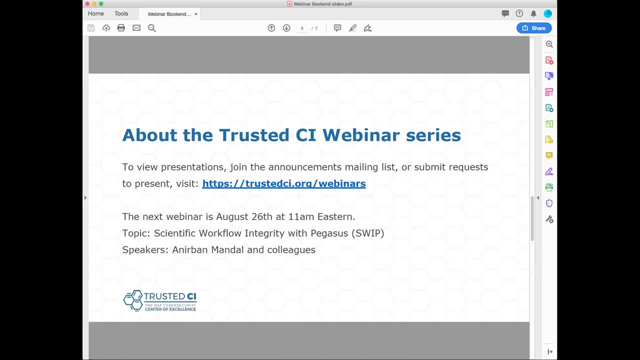 Have you explored any examples using healthcare-oriented apps like Step Monitor or Heart Rate Monitor? Yeah, that's exactly. you know an area where I think ANSILE can fit. you know really, really well. So there's another project going on inside of Cornell Tech. 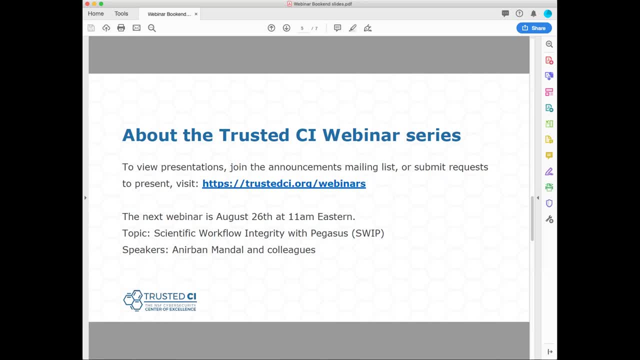 that uses Google takeout, So for retrospective learning. this project is called Riddle And they're basically. the idea here is is that you kind of sync up Google takeout and it dumps a bunch of your data and they can do some retrospective learning to, to get some kind of 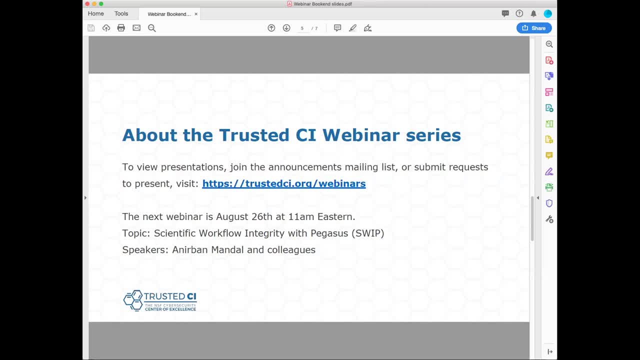 greater population sized insights about health and wellbeing, about depression, about a whole bunch of different areas, And so right now there's actually a study going on using that data and they're actually doing a formal study about that. They're not using ANSILE right now, but this would 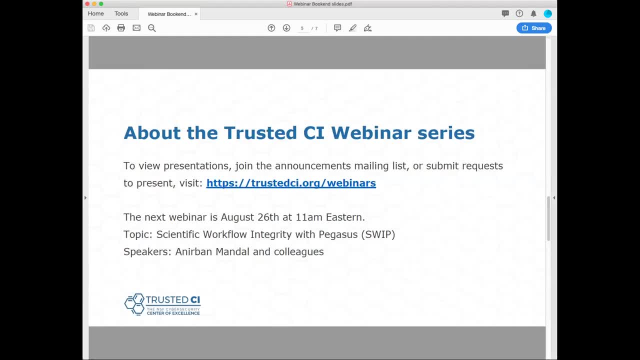 be a perfect use case, And so the next thing that we're exploring is: is that, what would, what would a ANSILE version of this study look like? Is our policy language flexible enough to support that? And we can, you know, can we do that? But the whole area of step monitoring and 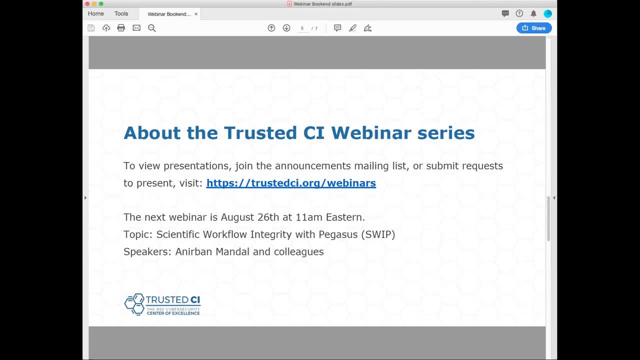 health and wellbeing is a whole different area, And so the next thing that we're exploring is is definitely, I think, a very good fit for ANSILE, And we really want to move in that direction. I've got another question here: How much flexibility does the data owner have for? 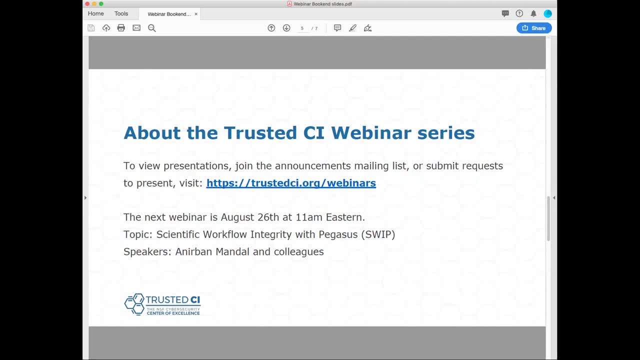 setting data access policies via ANSILE web. It appears the program that runs in ANSILE core needs to be aware of each policy condition, So policy changes would require changes to the program in ANSILE core. Yeah, So there's. 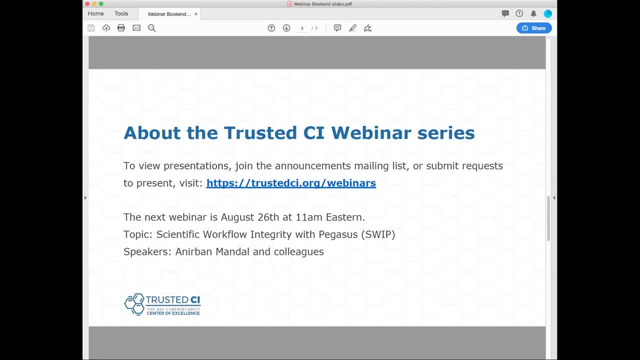 there's definitely a lot of flexibility there And I think that's a good fit for ANSILE. Definitely a relationship between the program and and the policy. right, You can't necessarily write an effective program without having some understanding of of the policy. There's a couple. 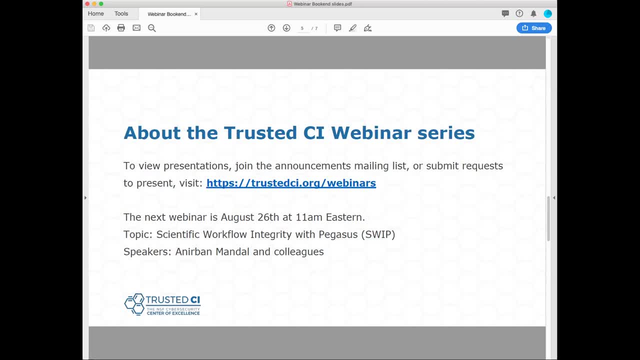 of ways I think we can go about that. So right now kind of our model is is that end users aren't necessarily going to be setting the policy, The, the, the envision, though we give them the flexibility to do that, But right now we're not necessarily going to be setting the policy. 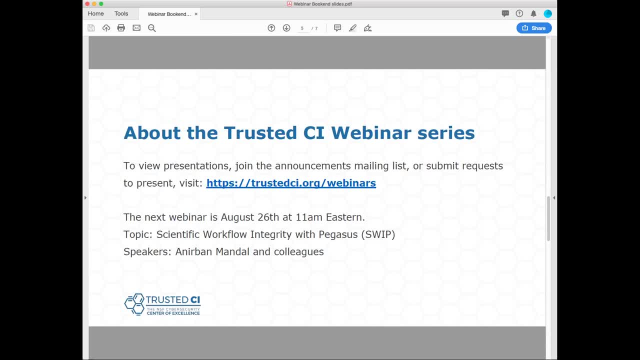 So right now kind of our model is is is that we have kind of policy administrators. So you think of this as someone you know, a PI on a project, someone who is, you know, maintaining the IRB, And so in that case, right, if you have kind of IRB sort of things, you probably only support. 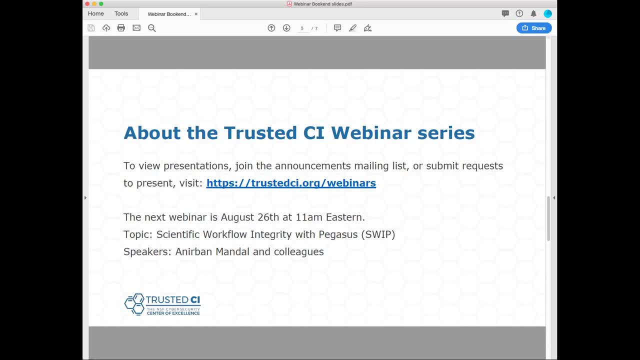 one policy that the user can really either, if you're going to participate in the study, here is the policy- Or we anticipate, you know, giving the users a small number of choices, Like here are kind of you know, a couple of different choices, not kind of an infinite number of that, But what we do though. 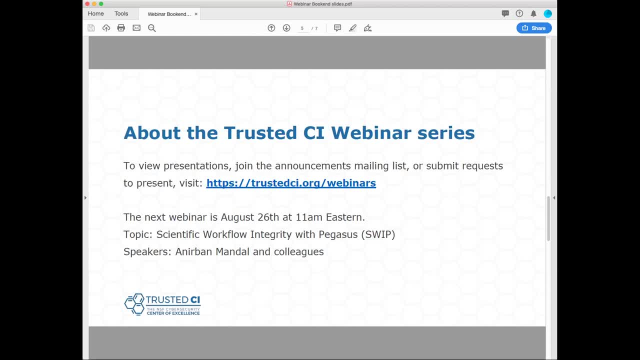 is applications. through a request into into ANSILE, they can get the specific privacy policy associated So you could dynamically look at what that policy is and construct your program around that. The person responded: thanks, So we've got. we've got three questions up here. 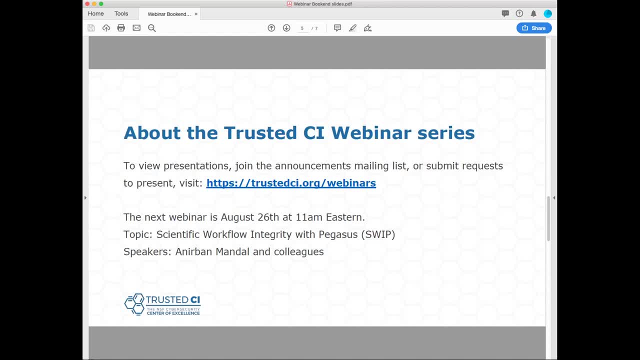 So I will do the. I'll just run through them and then let you answer after each question, after I read each question. So, question one: who are your customers, app developers or end users of the apps applications? Sure, And in some ways I kind of think both. 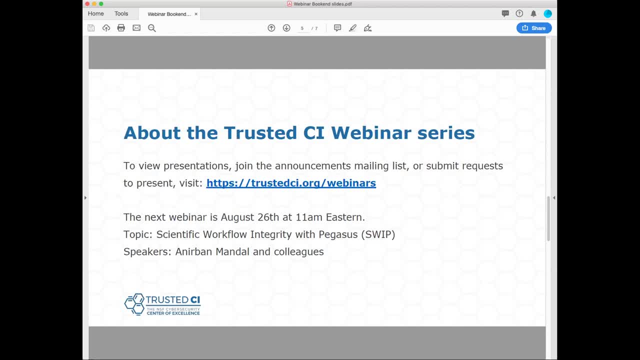 you know. so in some sense, you know, we want to make ANSILE attractive such that application developers would want to use it. So we want to make it attractive such that application developers would want to use it. Right, Because in some sense, you know, I like to think of ANSILE is helping applications do the 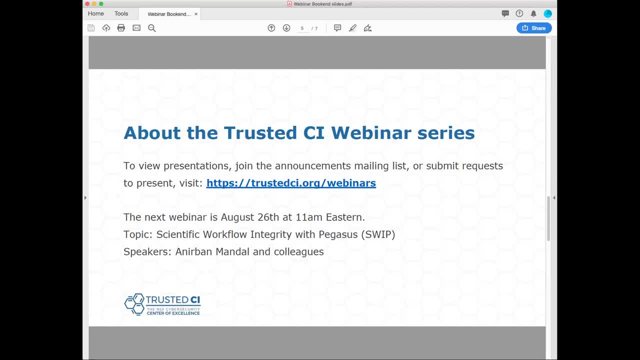 right thing, Because you could- you know there's either it. so I think there's a couple places, So one- you could kind of work in a semi-closed environment, So kind of you know. that's what I'm thinking kind of like a campus planning, enterprise planning, where you say, oh, here. 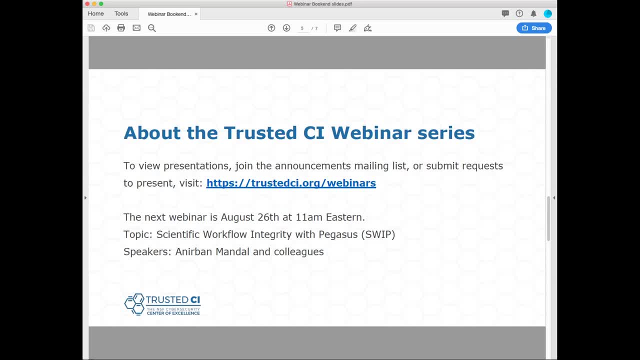 here's this application. You know we're going to use this. It's going to monitor your location, but we put these safeguards in place to do this. you know we're only going to use it in these very specific enterprise specific manner. So in some sense, right, we're trying to. 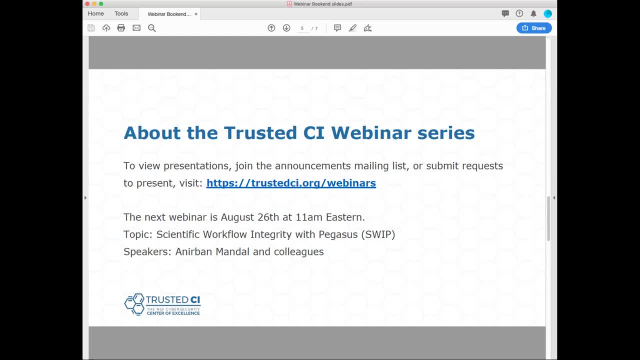 create a robust environment that application developers would want to use- ANSILE And- but you know, end users too. we want to make sure that they feel empowered to use these applications and that they have some faith and trust That these applications are doing what they say they're doing. 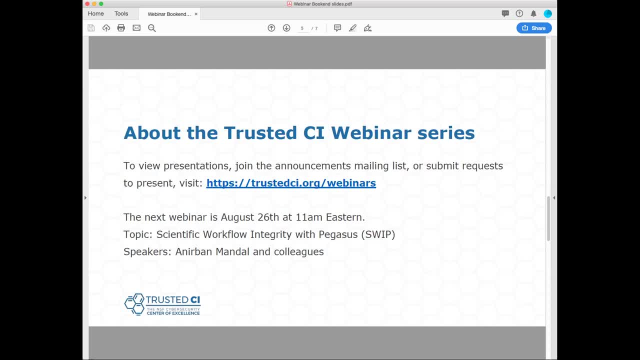 Okay, next question. Let's say an app's intention of collecting location data is not bad, So they would simply apply those filters to insert noise in the location data. Why would they enroll something like ANSILE, In other words, if the app developers wants to want to know the exact? 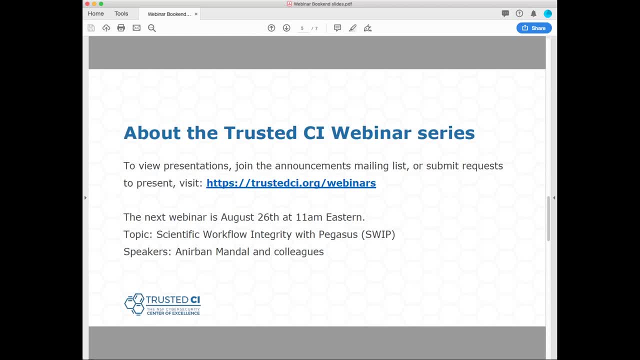 location. why would they agree to use ANSILE? Let's see, I think I missed some of that, but I can see the chat, So let's say so an app is okay, so the app is. we're assuming that the app is trusted in this case, And so I guess the question. So I 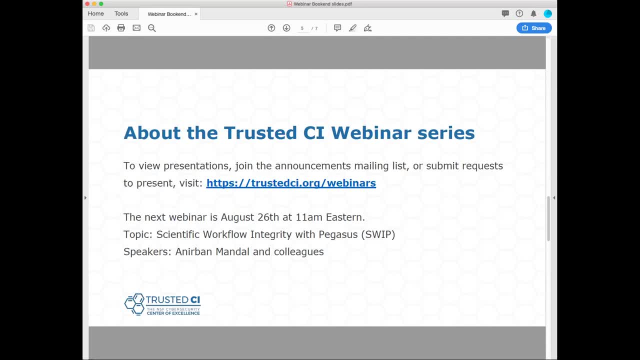 think the question gets to where is that computation being done? Right? So if we trust the application, then I don't know that the overhead of you know moving the computation inside of ANSILE is worth it when we can simply get the location data directly from there. So I don't. 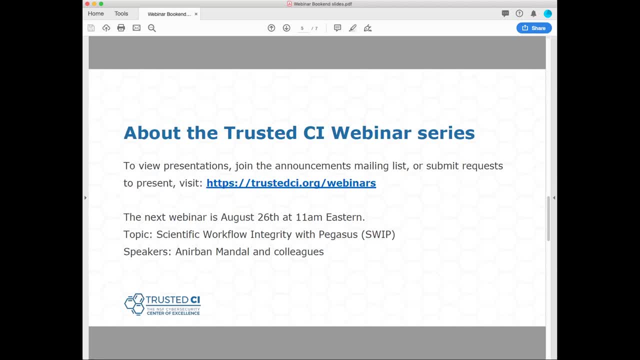 think it. you know, I think, if you trust the app- and I think that's a big if, I think that you know, doesn't? you know it mitigates the need to use ANSILE, but that's, I think that's a big if. 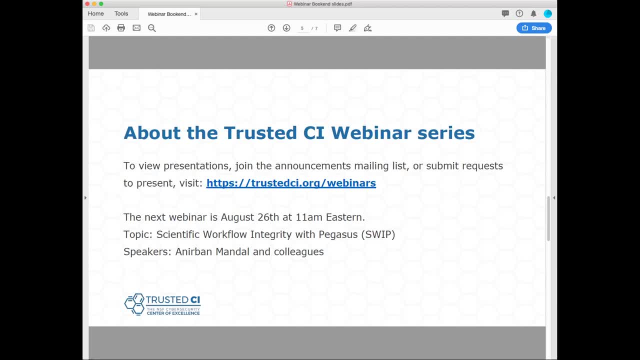 And then the third question: can you briefly explain the workflow and data flow? if I want to use ANSILE on my phone, Sure, and I think probably the best way to do it is kind of thinking about that kind of workflow. I did through the at the beginning. So ANSILE is a web service, so all of 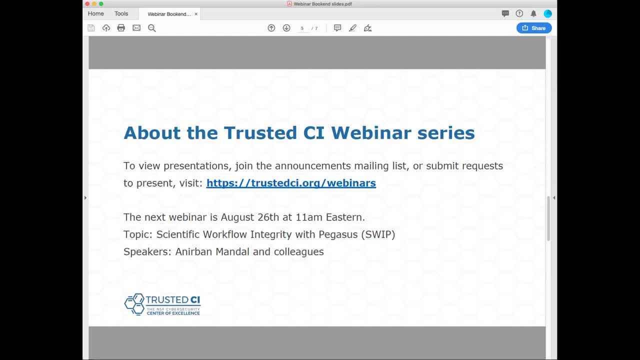 these requests come in through HTTPS, and so if your application wants to request ANSILE, you can request it through HTTPS. So if your application wants to request ANSILE, you can request it through HTTPS. So if your application wants to request some data from ANSILE, it would just make the 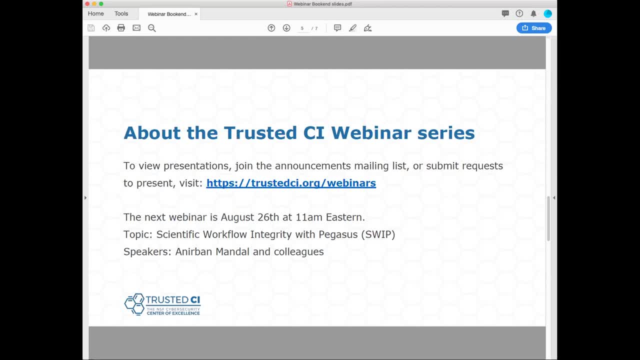 HTTP request with the program that would execute inside ANSILE the users you know associated with that, you know with that request, and then what comes back? a response comes back And I didn't get into that, it's just too many details, but the response that comes back is an. 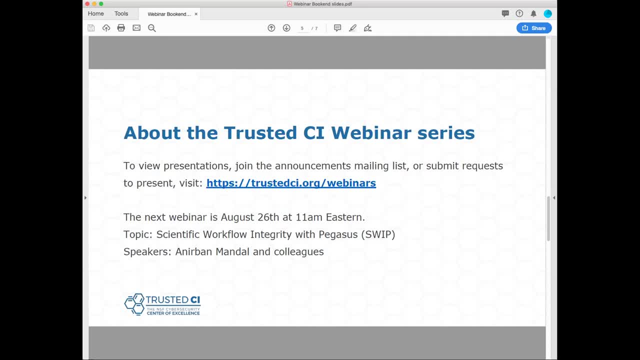 HTTP, you know, is a response that has the data associated with it. if there was any errors, right. if the request had failed, it gives you some errors for debugging information. So a mobile phone app just needs to make an HTTP request. 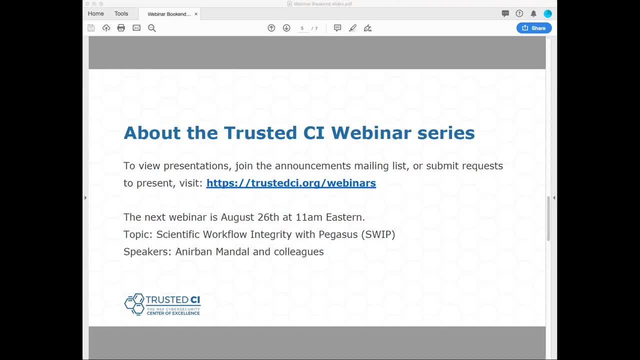 Okay, let's see if we get any replies to that series of questions. Why don't we start doing our last call for questions, because we're kind of coming up on the top of the hour. Oh, here's the reply. So both the users as well as the app developers have to register with. 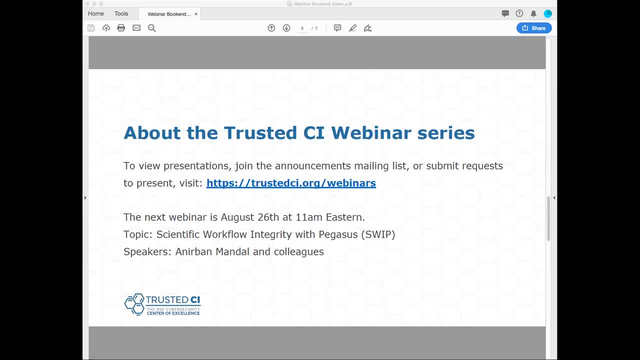 ANSILE. That's correct, right, So I didn't show the app interface, the web interface to ANSILE. but they register their app and they get a. you know, they get a secret token to verify that the app is who they say it is, and then users again go through that process And so